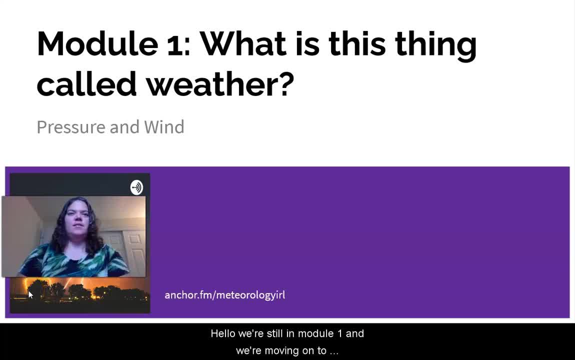 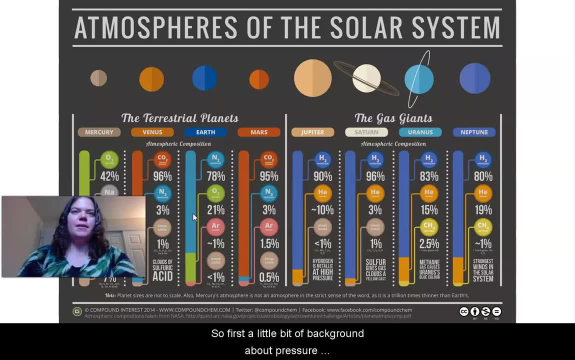 Hello, we're still in module one and we're moving on to lesson five, which is pressure and wind. So first a little bit of background about pressure. I wanted to give you the atmospheres of the solar system. So here's earth in the middle and our atmosphere composition is mostly nitrogen. 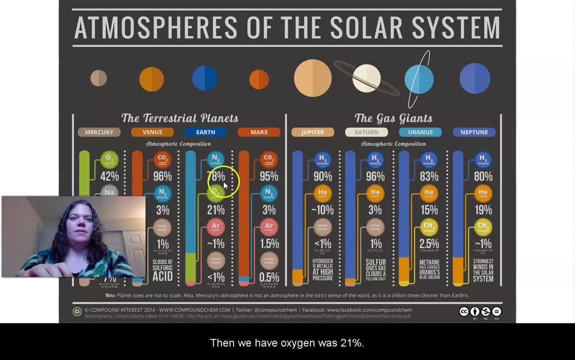 which is the blue component here. Then we have oxygen, which is 21%, and then argon and other various gases. Now, when we compare to the other planets in the solar system, you see that both Mars and Venus have a large component of CO2, which is carbon dioxide. 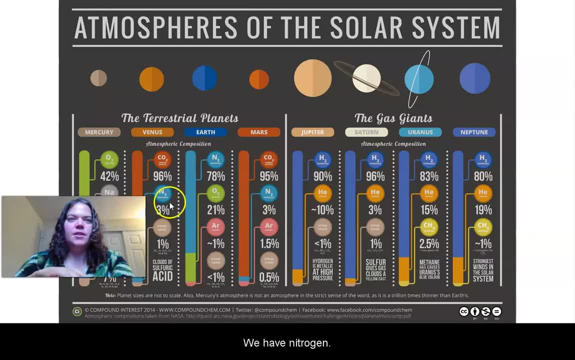 And then we have nitrogen and then other various gases, And mercury is mostly oxygen, but it still has a thin atmosphere, as well as Mars, And then the gas giants generally have mostly hydrogen. So our planet is the, as they call it, the Goldilocks planet. It is perfect. 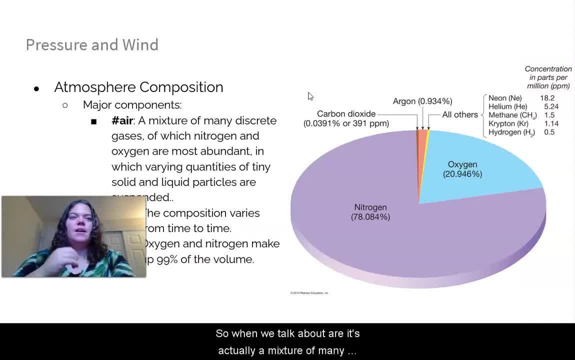 for sustaining life. So when we talk about air, it's actually a mixture of many discrete gases, of which, like I just said, nitrogen is the most abundant, So it's 78%. And then we have hydrogen, which is the most abundant, So it's 78%. 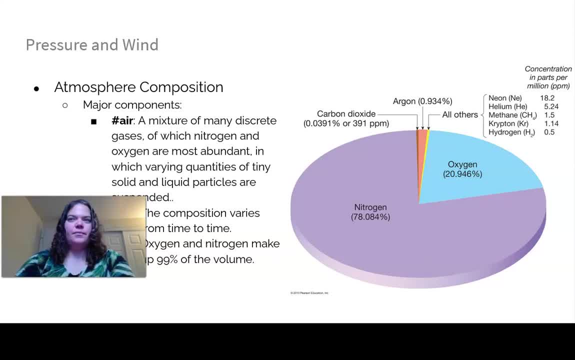 So it's 78% of the dry air, And then oxygen is 21%, And everything else falls into that smaller category. So please note that carbon dioxide is 0.04%. Of course this number is changing. And then we have argon- that's the third most abundant gas, And then everything else. 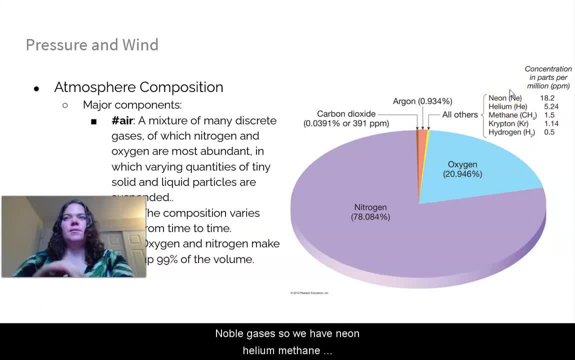 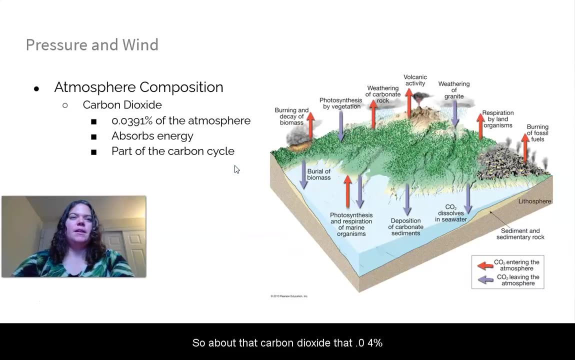 these are our noble gases. So we have neon, helium, methane, krypton and hydrogen, And the composition of these vary from time to time, And oxygen and nitrogen make up 99% of the total volume. So about that carbon dioxide, that 0.04% of the atmosphere? it is part of something. 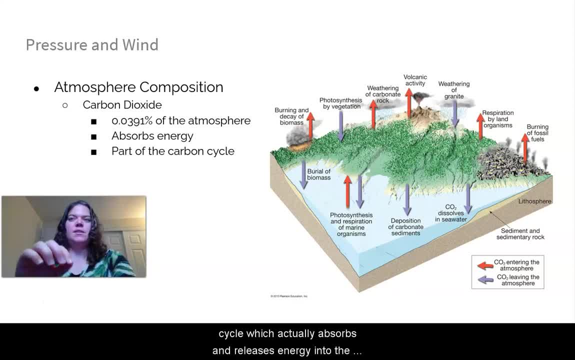 called the carbon cycle, which actually absorbs and releases energy into the atmosphere. So we see in this diagram- this is kind of a simplistic version of what the carbon cycle looks like- We see burning, which is the amount of carbon dioxide that is absorbed by the atmosphere. 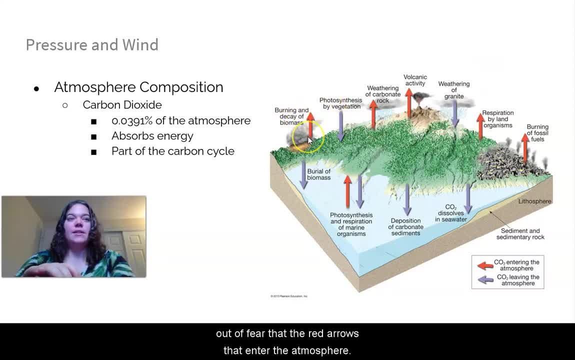 releases into the atmosphere. that's the red arrows that enter the atmosphere, and then the blue, purple arrows are leaving the atmosphere. so if we bury things that are biomass, that's going to leave the atmosphere. we have co2 that dissolves in seawater, um, and then the opposite is also true. 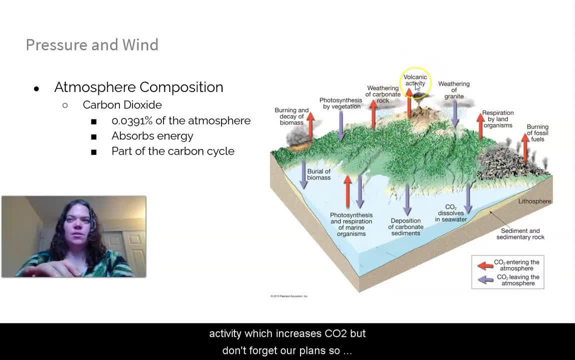 so we have volcanic activity, which increases co2, but don't forget our plants. so our plants increase photosynthesis and that will leave the atmosphere as well as marine organisms. so phytoplankton also takes up a bit of our co2, another greenhouse gas, that kind of surprises. 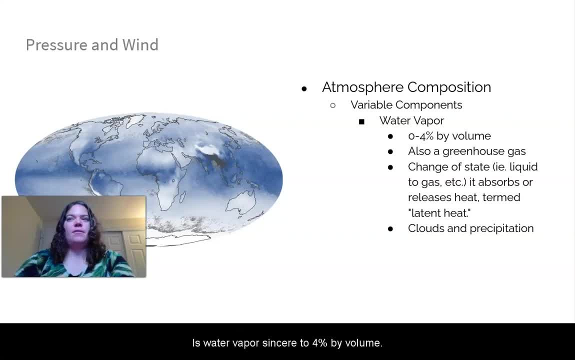 people is water vapor, so it's zero to four percent by volume, and the four percent would be kind of centered around the equator or the middle section of the planet, and then it goes less and less as we go forward to the poles. like i said, it's also a greenhouse gas. it changes state at normal temperatures and 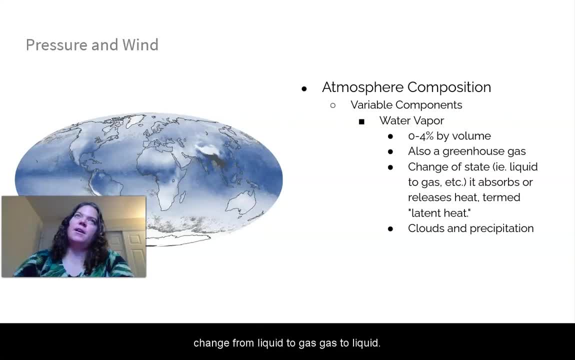 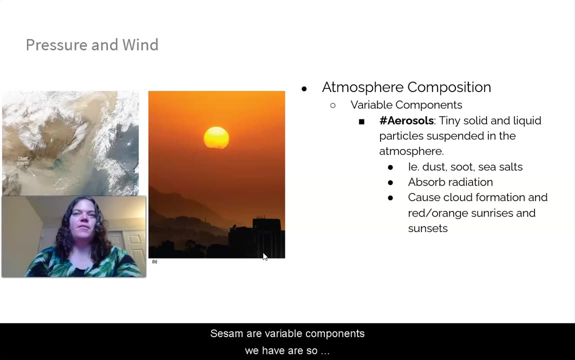 pressures, so it can change from liquid to gas, gas to liquid, liquid to solid and when that happens, it releases or absorbs something called latent heat, and this is what our clouds of precipitation is made out of. so some more variable components. we have aerosols. these are tiny, solid and liquid. 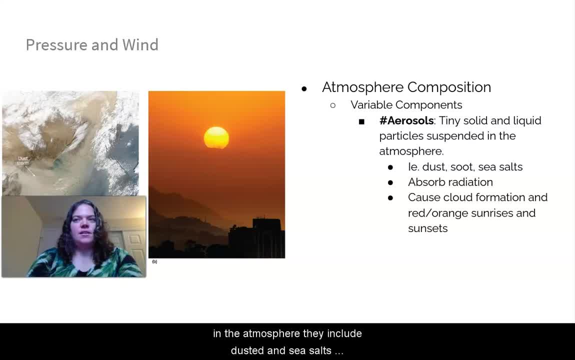 particles that are suspended in the atmosphere. they include dust, soot and sea salts. you can see some here making a red or orange sunset. now we do normally have red or orange sunsets, but they get a little bit more brilliant when we have more aerosols and these also absorb radiation. you can see here big dust storm, lots of air pollution. 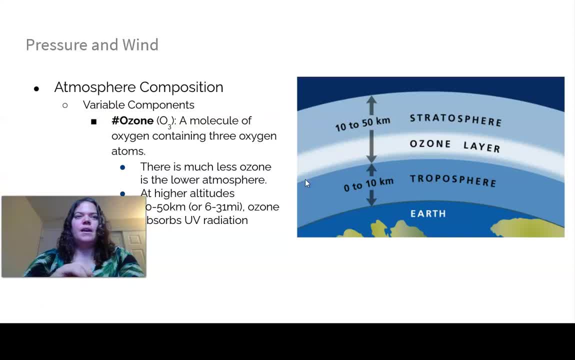 that's in asia. and then we have ozone. so this is o3. it is three oxygen atoms together and there's actually less ozone in the lower atmosphere. it is safer up here in the stratosphere. so we'll learn about this later in class. but the troposphere is the bottom layer of 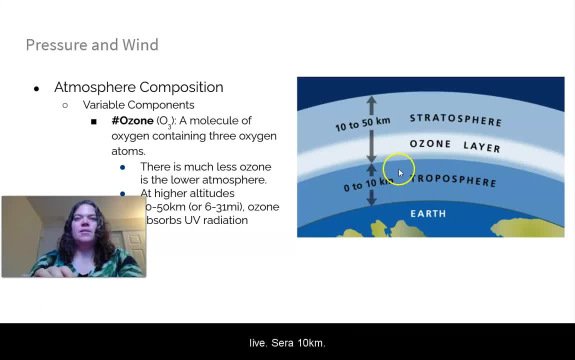 the atmosphere. that's where we live. it's about zero to ten kilometers or um up to six miles. well, six to ten sort of it varies um, but anyway. so the ozone layer protects us from uv radiation, so we want it to be up in the stratosphere, but when it comes to breathing it in, that's dangerous. 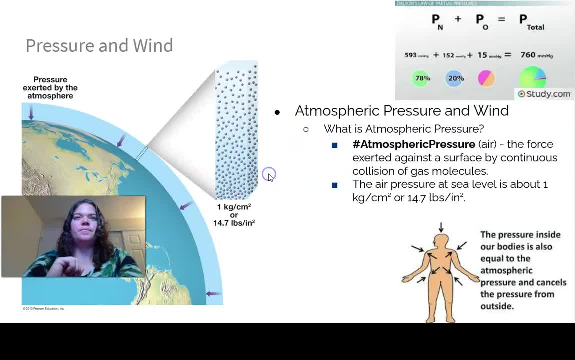 and we'll cover that in the air pollution chapter. okay, so what is atmospheric pressure? well, atmospheric pressure is by the air. it is the force exerted on a surface by continuous collision of gas molecules. so that surface could be your skin right, or it could be the surface of the ground, or a tree or an animal. what have you? so the air pressure at sea level is about zero to ten kilometers, about one kilogram per cubic centimeter or about 15 pounds per square inch. and how that works is our bodies actually give an equal pressure off, so the pressure is pushing in on us. our bodies push. 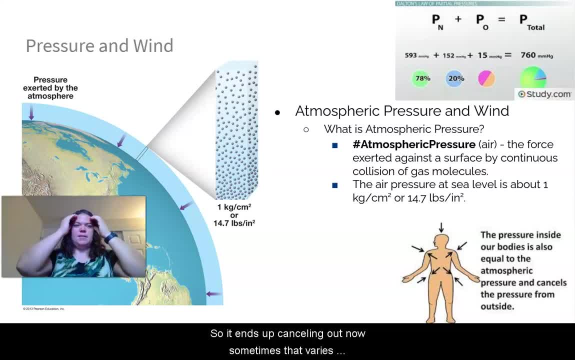 out, so it ends up canceling out. now, sometimes that varies and the pressure might be more extreme. so then your body aches, which we'll talk about later in the the weather and your health lesson. so when i talk about total air pressure, i'm talking about the pressure of each individual. 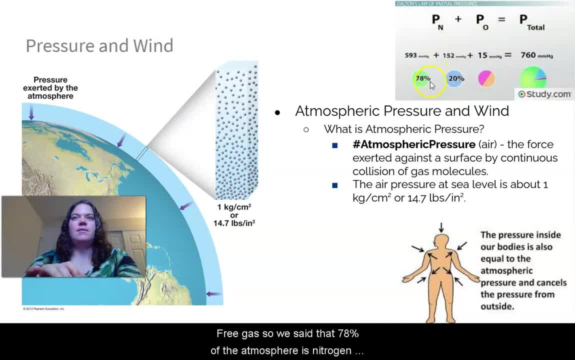 pressure um for each gas. so we said that 78 of the atmosphere is nitrogen. so we have a nitrogen pressure plus the oxygen pressure, plus argon plus blah blah blah equals our pressure total. so that's how that works. and then, when i'm talking about the continuous gas molecules, 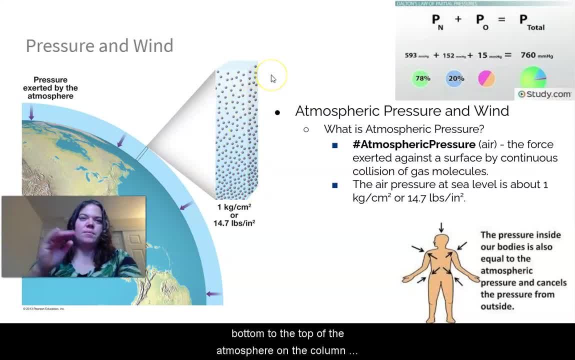 exerted on a surface. these are all those gas molecules that are in the atmosphere. so it's from the bottom to the top of the atmosphere, all in the column, that force all the way downwards. that's what we're talking about when it comes to pressure. so how do i measure it? pressure? 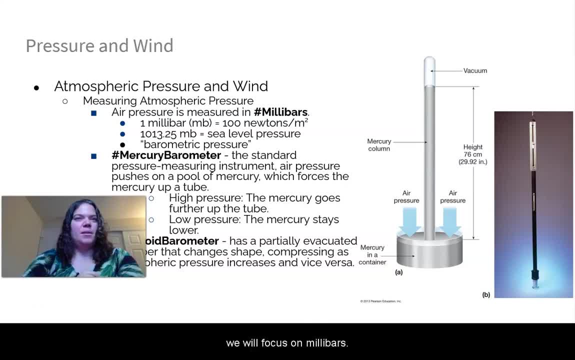 is measured in many things, but in this class we will focus on millibars. so a millibar is 100 newton square meter. you don't really need to know that, but in case you're interested. and for millibars, the average sea level pressure in the united states is ten thirteen point two five. 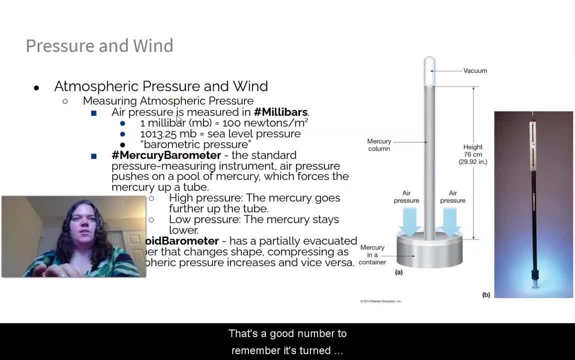 millibars. that's a good number to remember. it's termed barometric pressure because of this thing. so this thing is called a mercury barometer. it is a standard pressure measuring instrument. so the air pressure pulls, it pushes down on this pool of mercury in a container, which then forces. 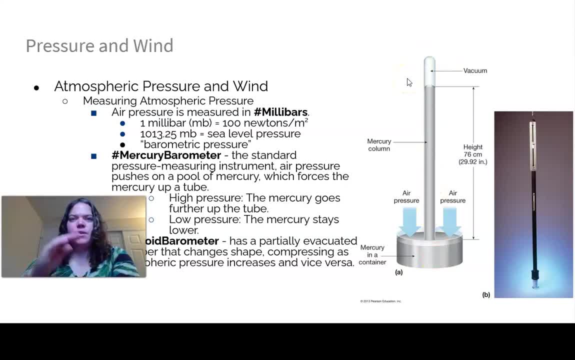 it to go up this tube, which has a vacuum at the top. so as it pushes more we get a higher pressure and it further fills up the tube, and that was called inches of mercury, so it's literally like from top of the pool to the top of the tube. that was the height in inches. 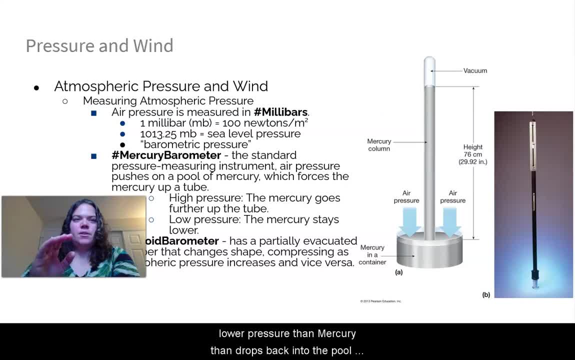 of mercury and then, as there's lower pressure, the mercury then drops back into the pool, so it stays lower. there's also an aneroid barometer, which I have a picture in a second. it has a partially evacuated chamber that changes shape, compressing and expanding as our atmospheric pressure changes. 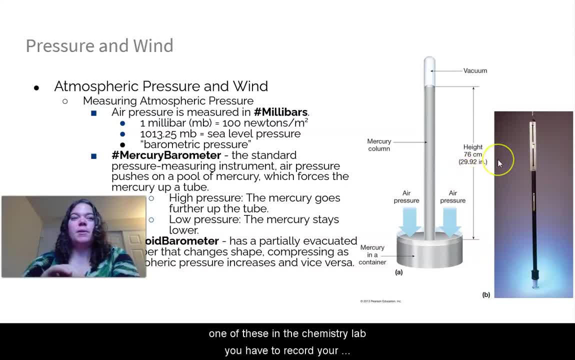 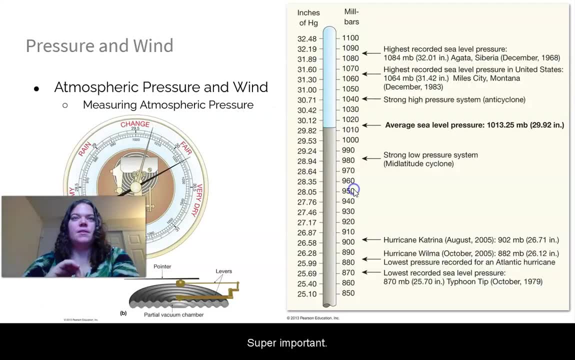 now you might see one of these in the chemistry lab. you have to record your pressure during chemistry measurements because if the pressure changes you might get different results. super important. so there's that aneroid barometer right there with the partial vacuum chamber and these are usually in these fancy guys here you see these in like gift um, what do they call? 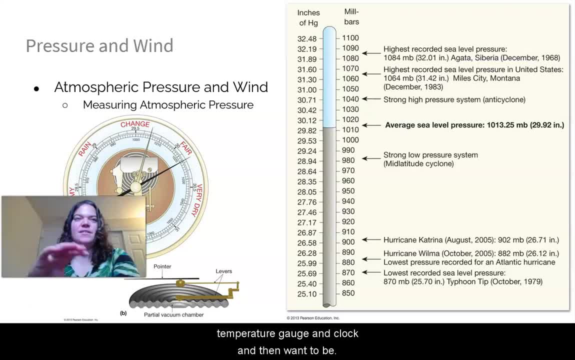 it. they're like in gift catalogs, so you have like a temperature gauge, a clock, and then one of these, and it tells you if it's going to change from stormy to dry or dry to stormy or whatever, and this one happens to have numbers on the inside. 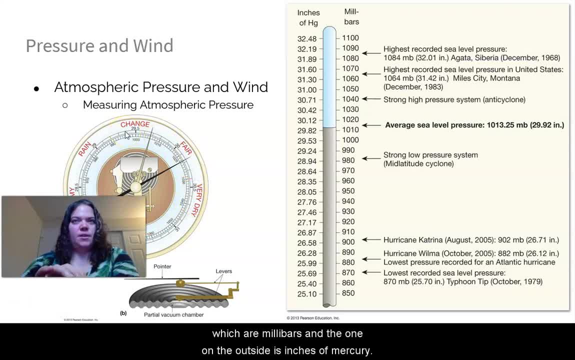 which are millibars and the one on the outside is inches of mercury. so I have a couple of um- I guess- points for you to know, so that you can know the extremes of pressure. so I'm going to start at the average here. uh, the end points, that's what we'll call it. so the end points of pressure. 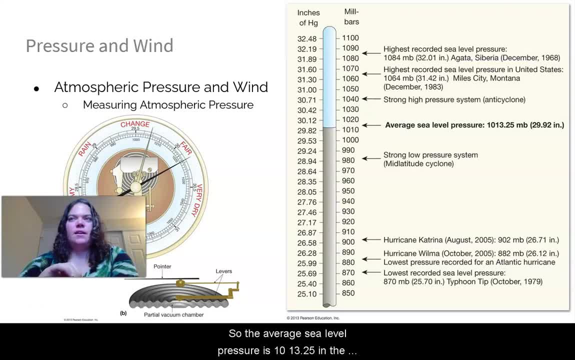 so the average sea level pressure is 10, 13.25 in the United States, which we've covered, or 29.92 to inches of mercury. now a strong low pressure systems of mid-latitude cyclone um would be about 980.. so then after that we have hurricanes, which Hurricane Katrina broke the 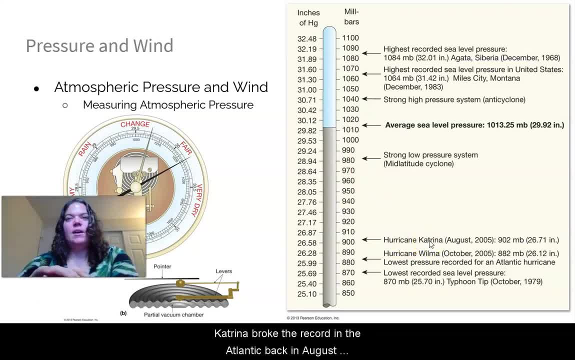 record in the Atlantic back in August 2005 with a low pressure of 902 millibars, and then Wilma the same year later in October, also broke the record. so now that is the lowest pressure recorded for an Atlantic hurricane, at 882 millibars. 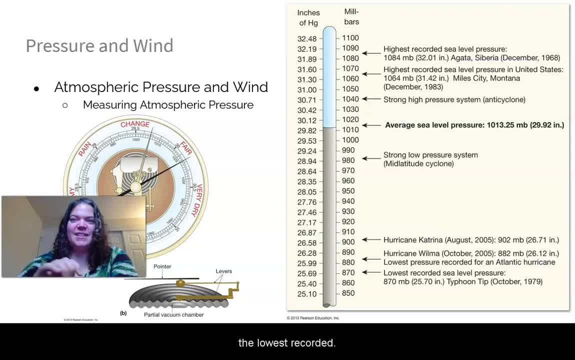 so that's very, very low pressure. and then the lowest recorded ever of ever is 870 millibars, which is typhoon tip in 1979.. go the other way. we see strong high pressure systems, or anti-cyclones, are about um 1040.. the highest recorded sea level pressure in the United States was 1064 in 1993 at 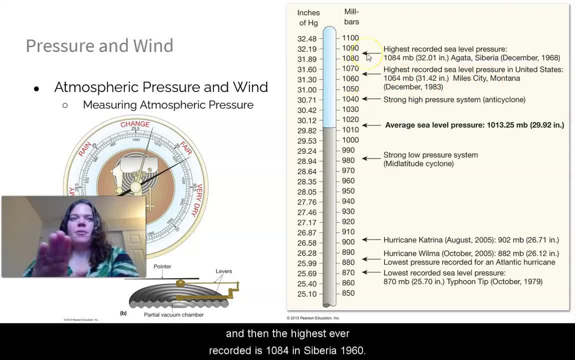 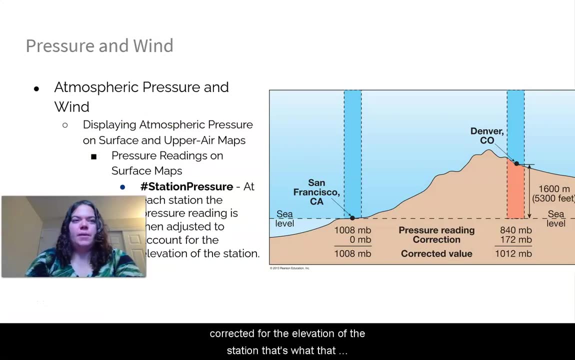 Mile City, Montana. so that's up here. and then the highest ever recorded is 10: 84 in Siberia, 1968.. that sounds very painful. so when I say station pressure, that's actually been corrected for the elevation of the station. that's what that means. so we both know, probably, that Denver is the 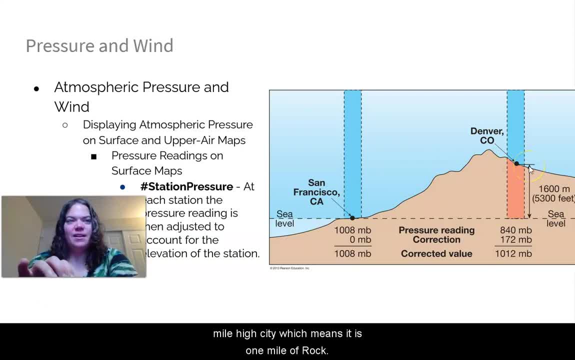 Mahai City, which means it is one mile of a rock above Sea level. right, so there's all of our mountain rock here. it's 5300 feet, or one mile, above sea level, and then san francisco is at sea level. so to get that difference, we just add: because pressure decreases with height increases, as you. 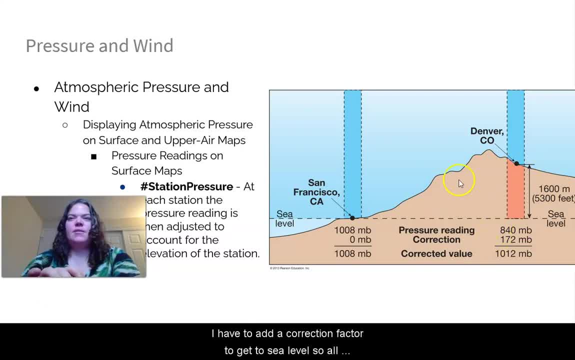 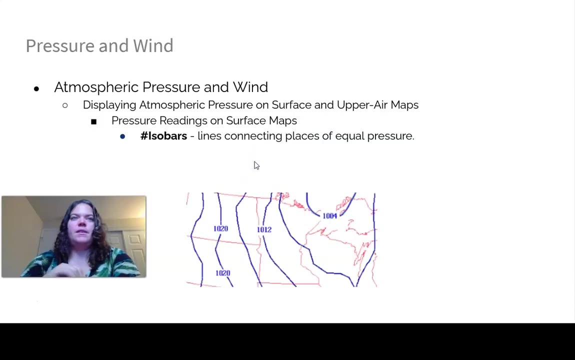 go down so i have to add a correction factor to get to sea level. so all the maps that we see that are surface pressure at, um, yeah, surface pressure. then they've been corrected to sea level based on the station's elevation. so that's the station pressure, okay. so when you see those maps that i 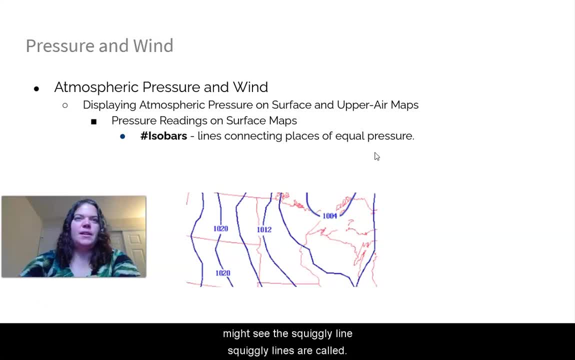 just referred to. you might see these squiggly lines. the squiggly lines are called isobars, so isobars are lines of connected equal pressure. so everywhere along this line is 1004 millibars. so it's been drawn by computers now, but it used to be drawn by hand. i had to draw by hand in undergrad. 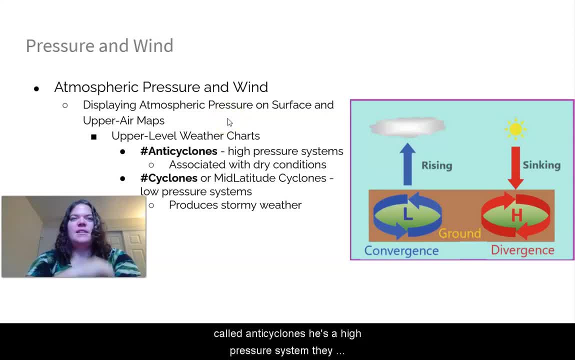 so on those upper level weather charts we'll see things called anti-cyclones. these are high pressure systems. they are associated with dry conditions, which we will get to why in a little bit later- and then cyclones or mid-latitude cyclones are low pressure systems and they 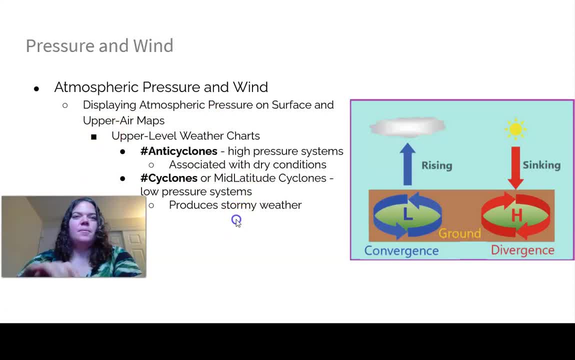 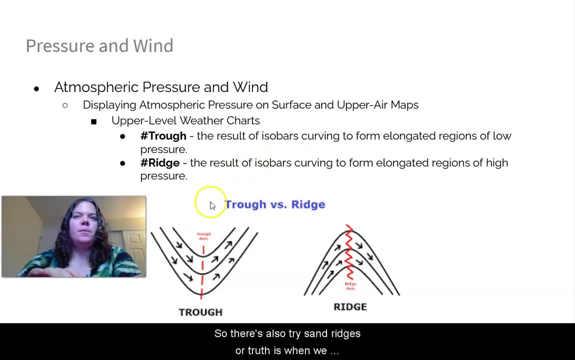 produce stormy weather, so move on. we'll get into more of those in a minute. so there's also troughs and ridges. so a trough is when we have isobars that curve um to form lower pressure, so they kind of look like a valley. 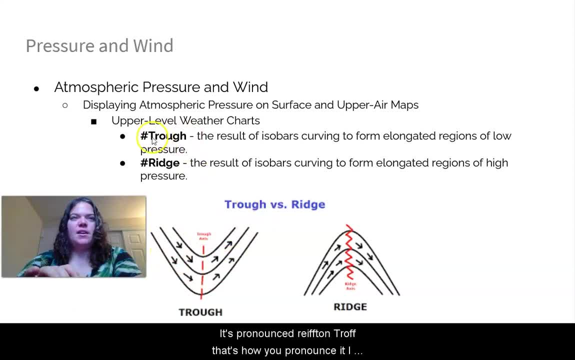 in the air. so here you go, that's a trough and it's pronounced trough t-r-o-f. trough. that's how we pronounce it. i know it's one of those weird words. and then ridge is on this side, so it kind of is like a mountain in the air. so this is high pressure, and when we talk about pressure changing, 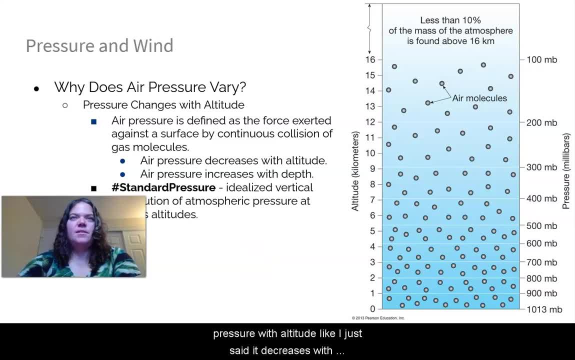 there are three ways it can change. so we have pressure with altitude. like i just said, it decreases with height right. so we see most of the air molecules here in the diagram on the right are focused towards the bottom and then they peter out as we go up. so the pressure should. 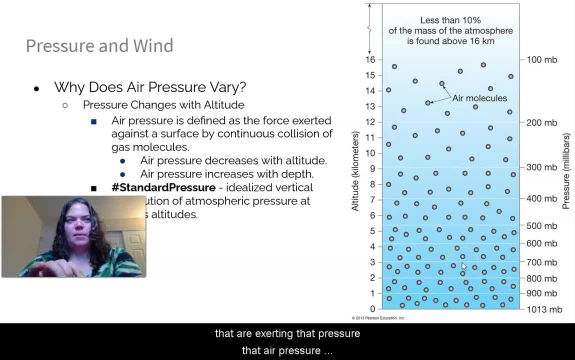 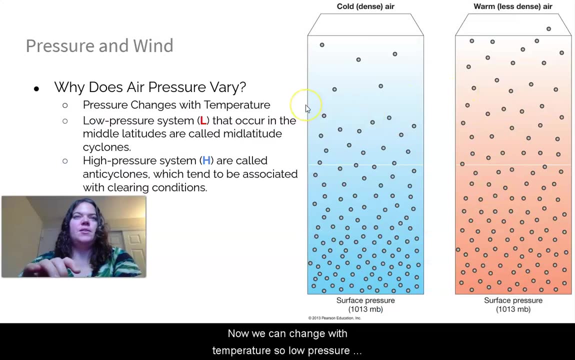 be more at the bottom because there's more molecules that are exerting that pressure. so air pressure decreases with altitude, increases with depth. this is the standard pressure and that's an idealized vertical distribution over atmospheric pressure at various. Now we can change with temperature, So low pressure systems are labeled as little red L's on maps, and high pressures are labeled. 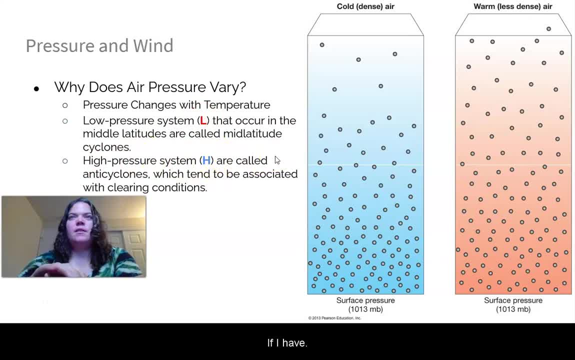 as blue H's. I just put that there for reference. But if I have cold, dense air versus warm, less dense air, this is what happens to my surface pressure. Oh, nothing. So what actually changes here? So you might expect, OK, well, the temperature is changing, so my pressure should change. 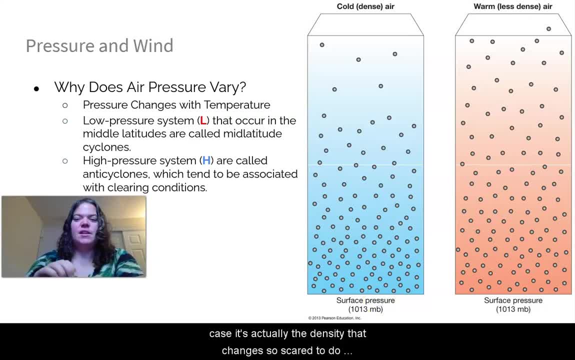 But actually that is not the case. It's actually the density that changes. So let's go through this. As I have cold air, you can think of it as like the air molecules get chilly, So they want to kind of crowd together to stay warm. 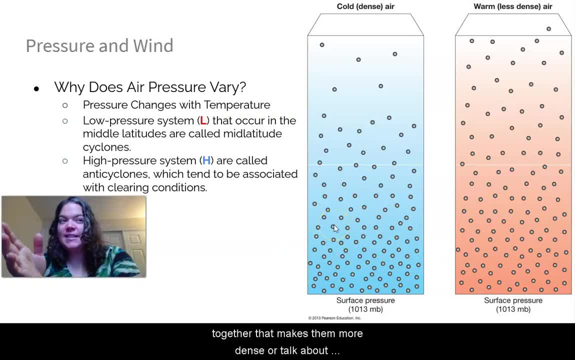 So here we see they kind of bunch up together. That makes them more dense. So we're talking about their density, not their pressure. their density, So you can think of: like the pressure is the weight Right, So I have the same weight. 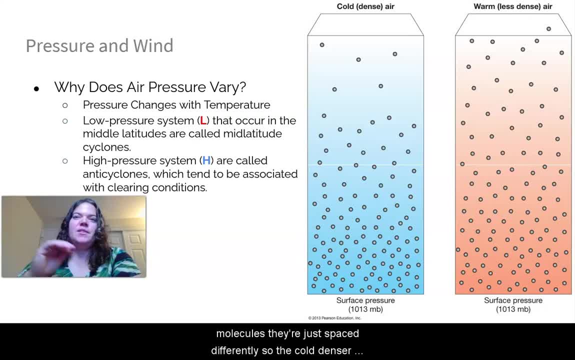 I have the same number of air molecules. They're just spaced differently. So the cold denser is kind of tightly packed, So they're more dense, And then the warm ones. it's like they're at the party and then they start dancing. 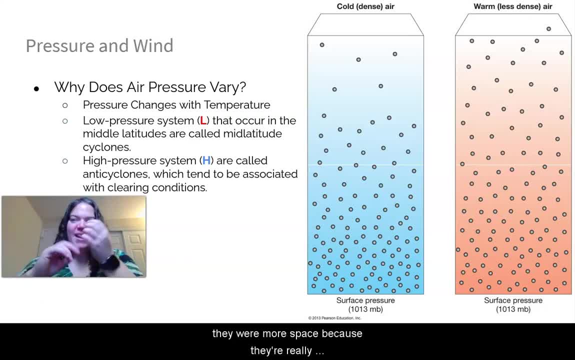 They have a little bit of BO, So they space out. They want more space, Right, Because everybody's starting to smell. Sorry, it's a bad metaphor, But anyway, you'll never forget it. So now they've spaced out. 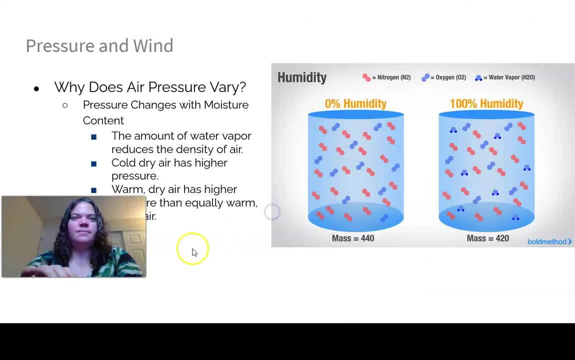 So this is warm, less dense air. OK. The last way it can change is through moisture content. This is the amount of water vapor that will then reduce the density of the air, Because why I'm taking out that portion of air and I'm replacing it with water vapor. 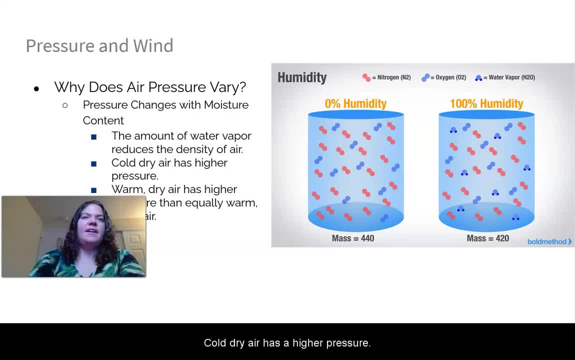 So the water vapor takes up space. So cold, dry air has a higher pressure. Warm dryer also has a higher pressure than equally warm and moist air. So the moist air means the density of the air decreases. So here you see: zero percent humidity. 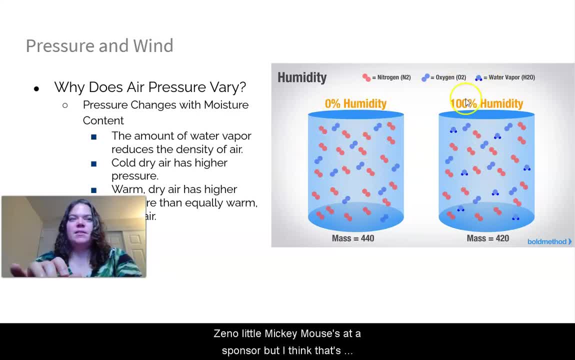 Right, We see no little Mickey mouses- not a sponsor, But I think that's what they look like: Little water vapor molecules. But when it's 100% we see much more little water vapor molecules And they take up space. 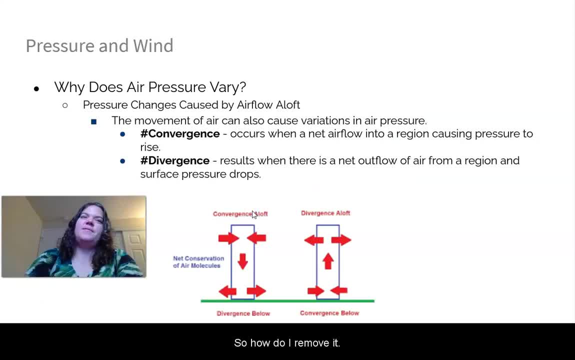 So that's why the pressure changes. OK, So how do I move it side to side, or up and down, or what have you? OK, there are two ways. we have conversions, which is a net inflow into a region. we have air coming together. air coming together, that's convergence, or the opposite, which is divergence, and then that is. 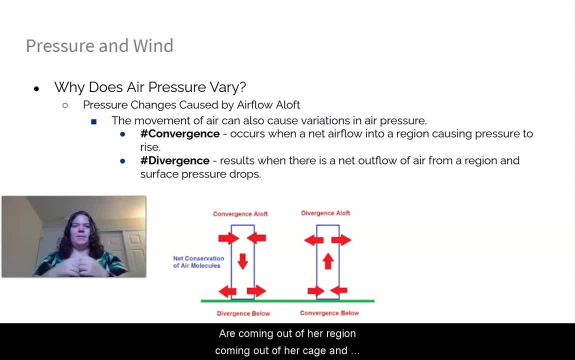 net airflow out, so i have air coming out of a region, coming out of a region, coming out of a region. so that's going to cause my surface pressure to drop, as opposed to the conversions, which causes it to rise because i'm piling up a bunch of air in one area. okay, hopefully that makes. 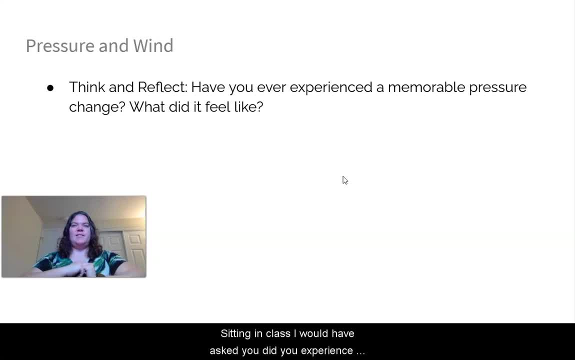 sense. so then in class i would have asked you: did you experience a memorable press or change? most people have been on an airplane at least once in their life and you have the ear pop kind of situation, so that's usually most people's experience. or going up the side of a mountain. 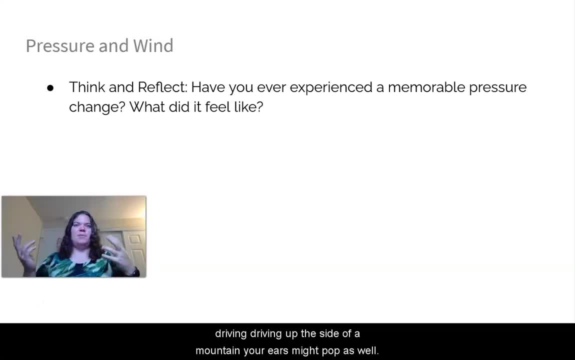 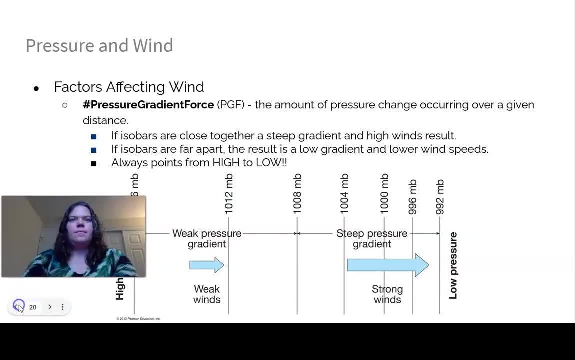 if you're driving, driving up the side of a mountain, your ears might pop as well. that's usually what what i hear in class. okay, so how do we generate any wind? so now we're going to put the pressure together with the wind. so to make my wind i need 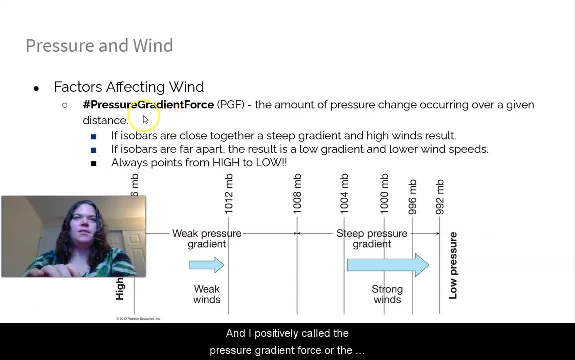 to have a difference in pressure and that causes something called the pressure gradient force or the pgf. that's what i'll call it from here on. so the pdf is the amount of pressure change over some given distance. the way you can tell is looking at your isobars, right the lines of equal pressure. 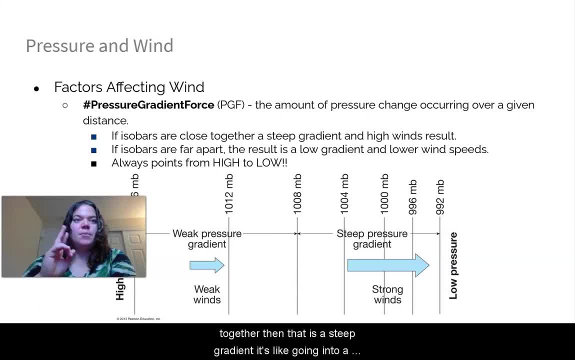 so if the isobars are close together, then that is a steep gradient. it's like going a valley. that's moving really really, really fast right, as opposed to if they're far apart. then i have a low gradient which leads to lower wind speeds. remember that the pgf always points. 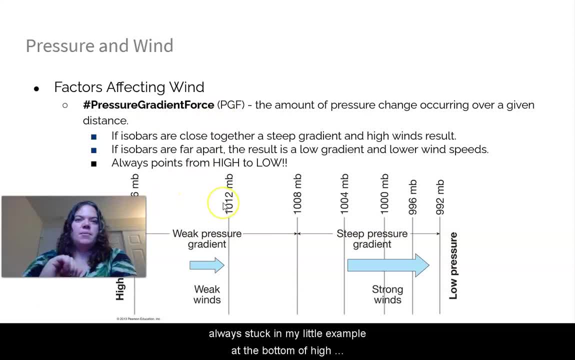 from high to low, always, always, always. so in my little example at the bottom we see the high pressure is on the left, which means pressure gradient force is always going to point to the right in this scenario, and i see my isobars here, so these are spaced every four millibars. so i see 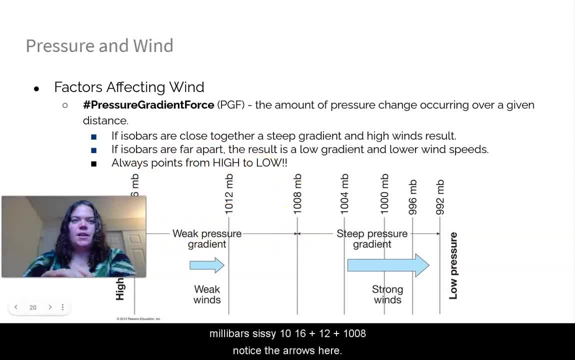 10, 12 and 1008. notice: the arrows here and the narrow arrows here are the same distance. okay, we're just supposed to trust them on that, but they're supposed to be the same distance. so between this distance i see a change of eight millibars, which is not a lot, so there's a weak. 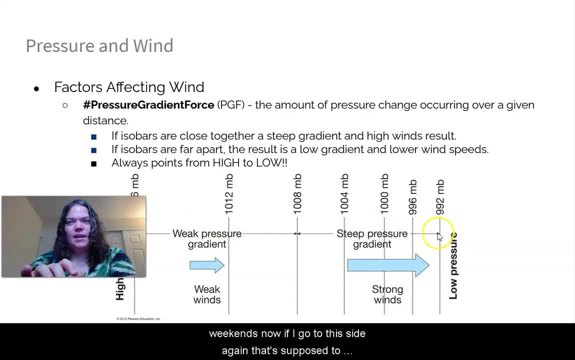 pressure gradient and weak rims. now if i go to this side again, that's supposed to be the same distance. it's like an optical illusion, but it's supposed to be the same distance. so if i go from to 992, let's see, that's the difference of eight. eight, so it's 16. it's doubled, so there's a double. 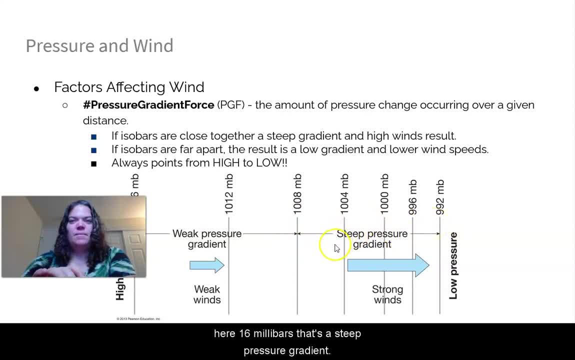 difference here 16 millibars. so that's a steep pressure gradient and there are strong winds. think of it as like when you put your thumb on the hose. if you have- i'm talking about a free flowing hose- okay, the water is squirting out, and then you put your thumb on it. 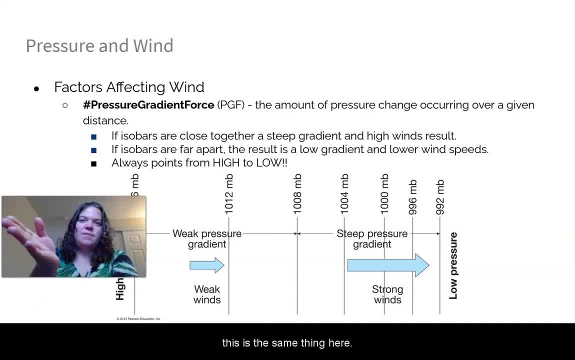 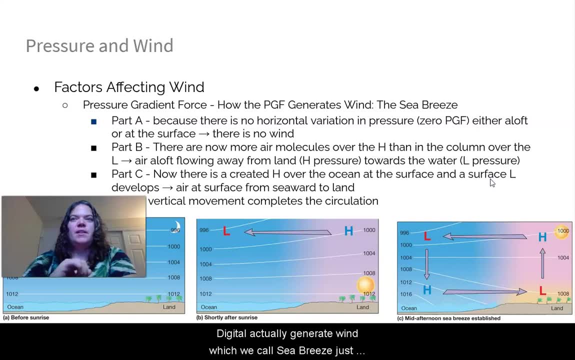 the water will squirt faster, right? this is the same thing here, right? oops, pgf will actually generate wind, which we call sea breeze. so just going through this example, in part a there is no horizontal variation because it's nighttime, so you see a little moon here it's. 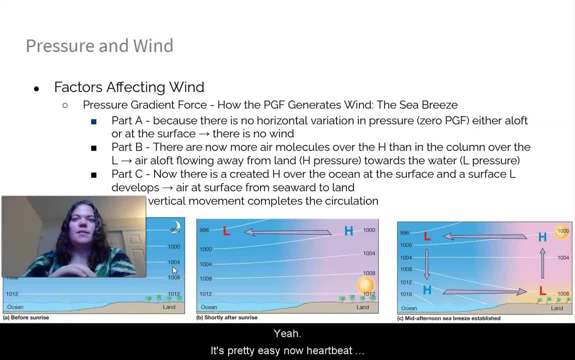 night there's zero pgf, there's no wind period. it's pretty easy. now, part b: after sunrise, we have more air molecules now over h, which is up here, then over l, which is over the ocean. so the air loft is going to point away from the grid, and when there 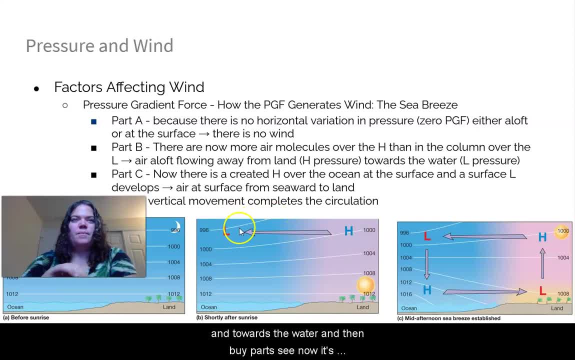 the land, remember, from high to low and towards the water, and then by part c. now it's mid-afternoon. there's been heating, the land is now hot so we have more um air rising from the surface of the land, not the ocean, the land- and so i see a little low pressure kind of develops over the land and 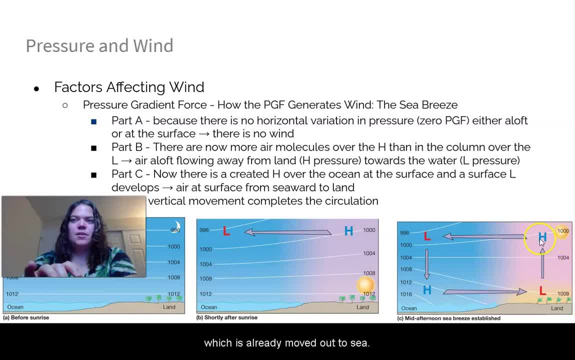 once that has happened, it's going to go up to the h, which is already moved out to c, and then it kind of gets replaced and it makes this little vertical um circulation, so it's kind of like a little circle, excuse me, um. so we see the little l of the land here and i i think you can see the little. 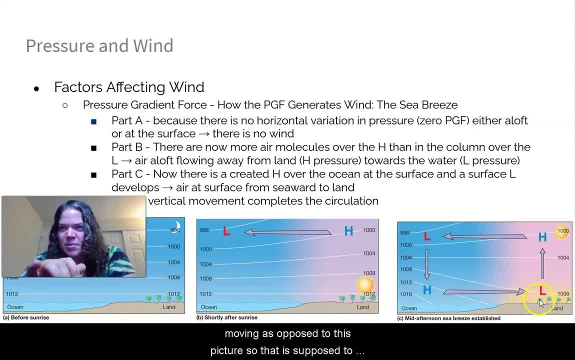 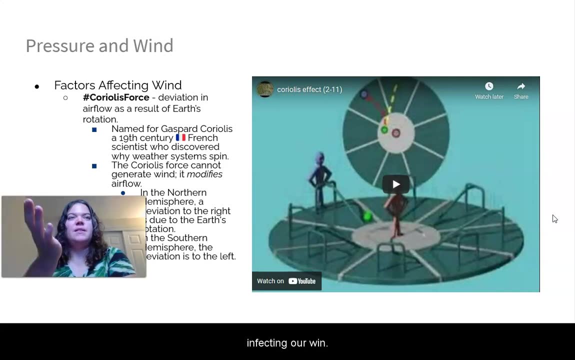 trees are moving, as opposed to this picture, so that is supposed to be the breeze coming from the ocean. okay, so because it comes from the ocean, it's called the sea breeze. we name things where they come from in meteorology. okay, so coriolis is the next force affecting our wind. this is a deviation in airflow, according to. 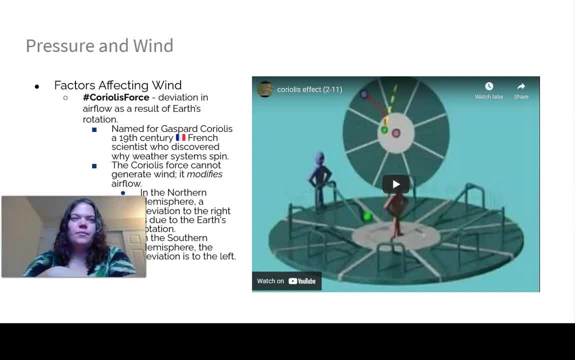 the results of earth's motion it was named for. gaspar coriolis was a 19th century french scientist- hence the little french flag- and he discovered why weather systems spin. if we were in class we would watch the video which kind of shows you why rotating causes this deflection. 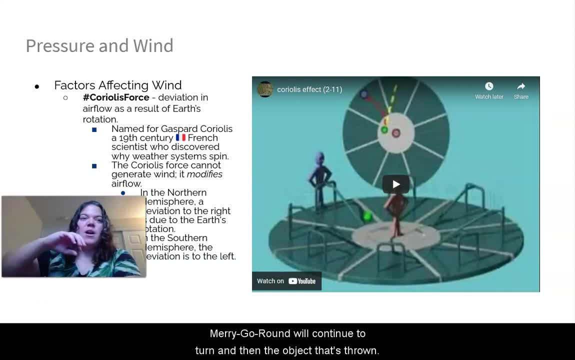 right, because the thing that you're on, whether it's the earth or this merry-go-round, will continue to turn, and then the object that's thrown, whether it's an air molecule or, in this case, a tennis ball, will move at a rate according to the air, not according to the ground. so it's. 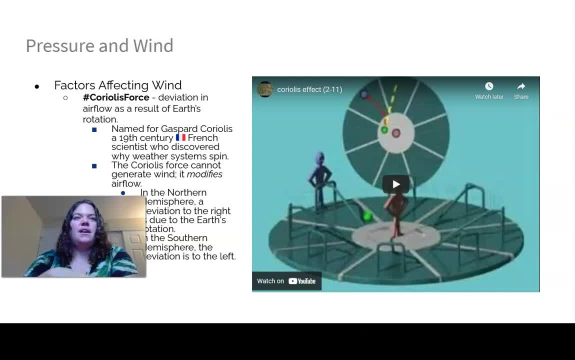 like relative motion, basically a little bit of physics, um, so it can't generate wind. the thing that generates wind is the pdf, okay, pressure, gradient force. this modifies the airflow. that's what happens. so in the northern hemisphere, this deviation is to the right because of the earth's rotation, and the southern hemisphere is to the left. now for the duration of this class, we 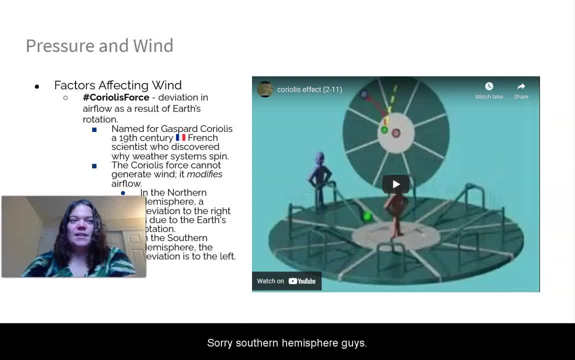 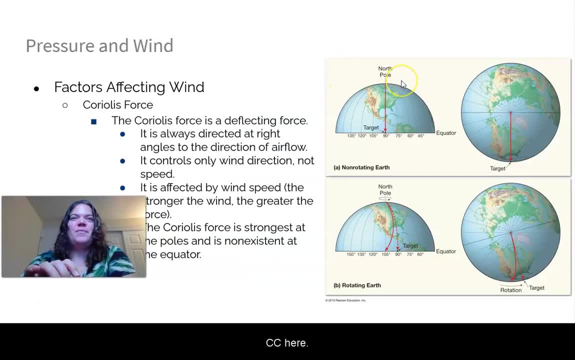 only talked about the northern hemisphere. sorry, southern hemisphere guys, but we only focus on the northern hemisphere in this class, okay? so you see here, if i'm at the north pole and i'm trying to target the equator, if i walk in a straight line on a non-rotating earth, so it's not spinning. 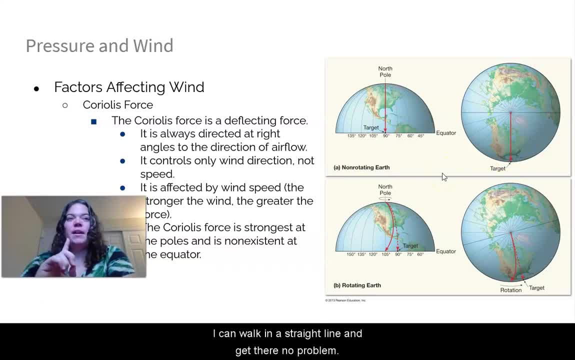 i can walk in a straight line and get there, no problem. but like i said, if i am at the north pole, i start the north pole. the earth is rotating like it normally does every 24 hours. then when i try to reach that target, i will be deflected to the right in the northern hemisphere, so i'll end up. 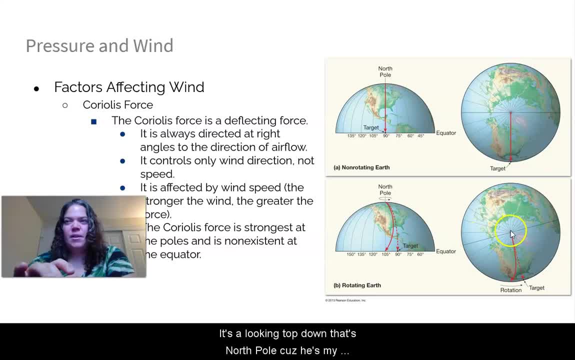 somewhere over here, right, so looking top down, that's north pole, so i see my target, and then, because there's rotating this way, i end up walking somewhere over there. okay, so again, it only changes the direction of the wind, not the speed. but if i have a stronger wind it will get deflected. 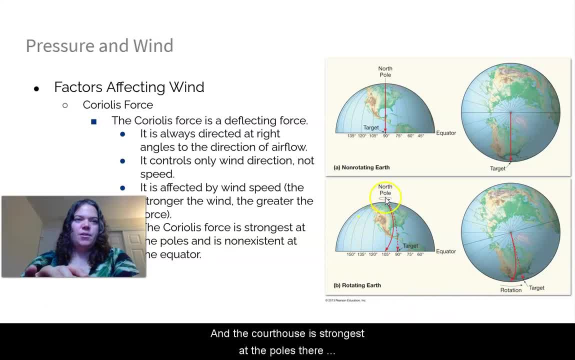 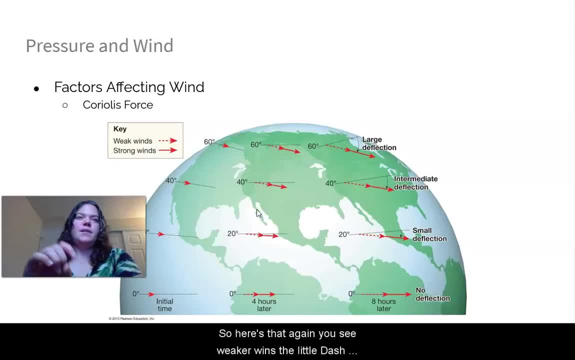 more, and the coreos is strongest at the poles, therefore, and non-existent at the equator, which will become important when we make our hurricanes later. so here's that again, we see weaker winds, the little dashed ones have a strong, a smaller, i'm sorry, smaller deflection as opposed to stronger. 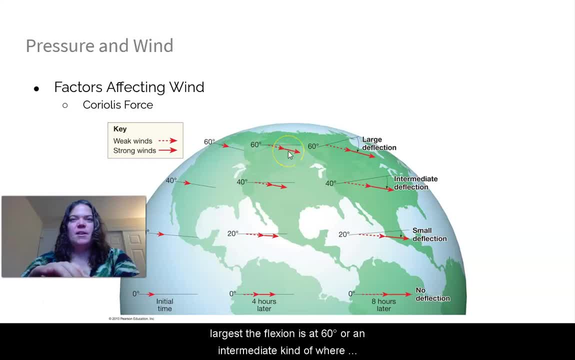 winds which give a larger deflection, as you can see over time. here the largest deflection is at 60 degrees or above, then an intermediate kind of where we are. this is why airplanes have to do like the arc thing because of that rotation underneath them just halfway up, and then smaller deflection at like 20 degrees. we're talking central. 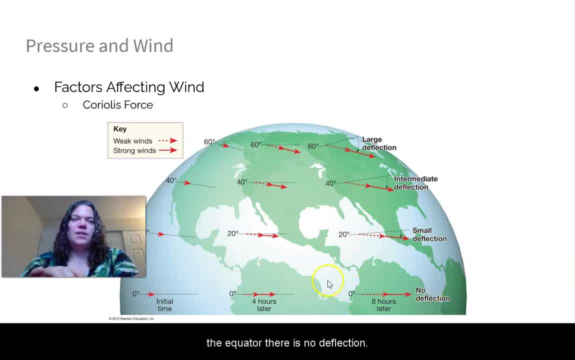 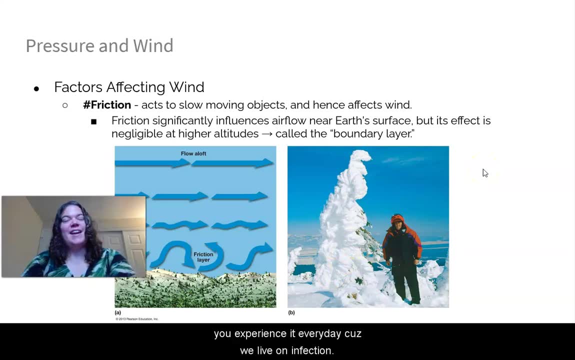 america now, and then, by the time we get to the equator, there is no deflection. now, the final force that acts on our wind is called friction. you experience it every day because we live on a friction planet. yeah, there's, there's friction on the planet. um, so it acts to slow. 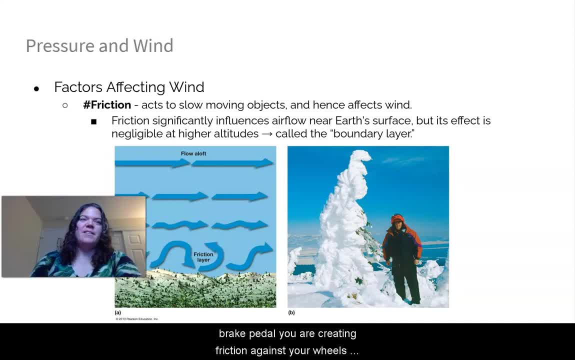 moving objects. so if you drive, when you press your brake pedal, you are creating friction against your wheels, using brake pads to try and slow and stop the vehicle. so in this case we're trying to slow or stop our wind and it significantly influences airflow in something called the boundary layer. so 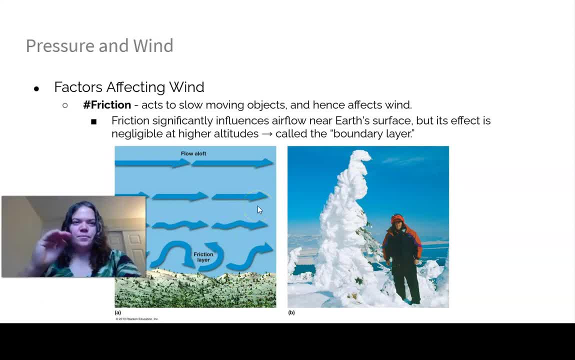 from here to the top of the area where friction no longer matters. that's called the boundary layer. so at higher altitudes, where we call glow a loft, friction actually doesn't matter, because at the surface we see trees and buildings and people and mountains in all kinds of other things. 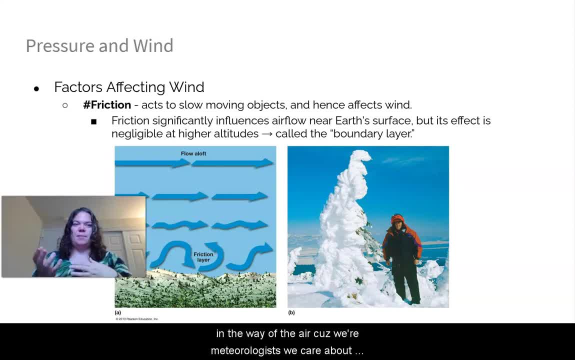 right that get in the way of the air, because we're meteorologists so we care about the air. so from the air's perspective, the mountains and such are in the way, so that's called the friction layer. then, um, when we get above that layer of the boundary layer, then we have no friction. so it's. 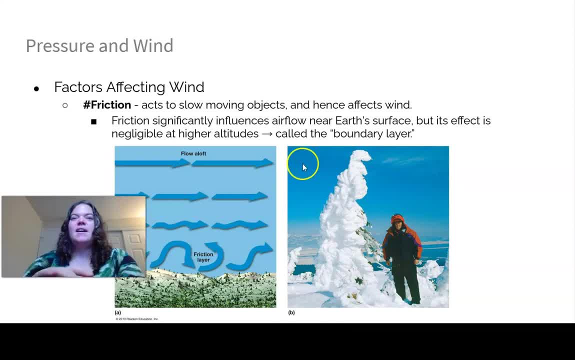 called negligible, meaning it doesn't matter. okay, so i put this picture here because it's in the textbook, but also because, you see, this tree here got in the way of the airflow, like i told you, so it kind of got sprayed with snow on one side, so how do i know which way the wind is? well, it. 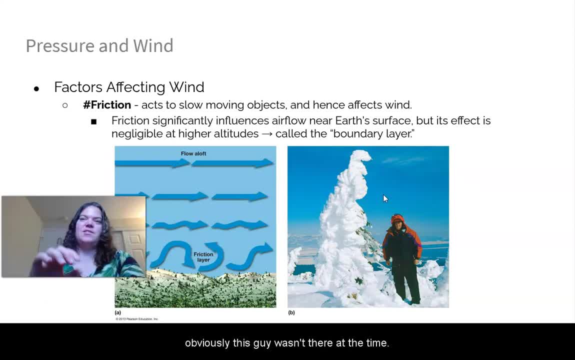 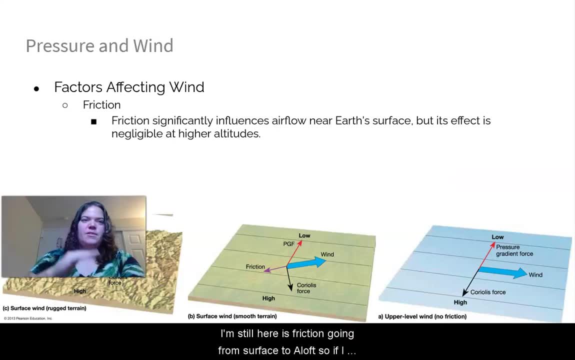 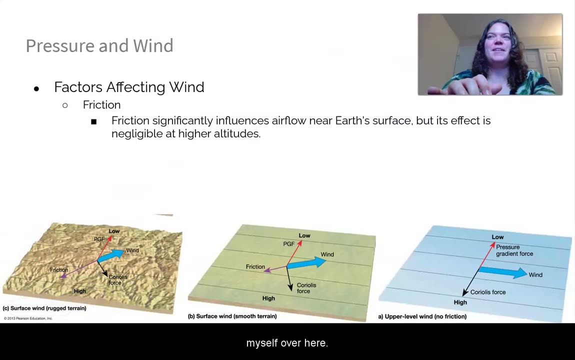 must have come from this direction, because the snow smashed into the tree, right? obviously this guy wasn't there at the time. all right, so here's friction um, going from surface to a loft. so if i start with the surface wind over here i'm gonna have to move me. so you can see, i'll put myself. 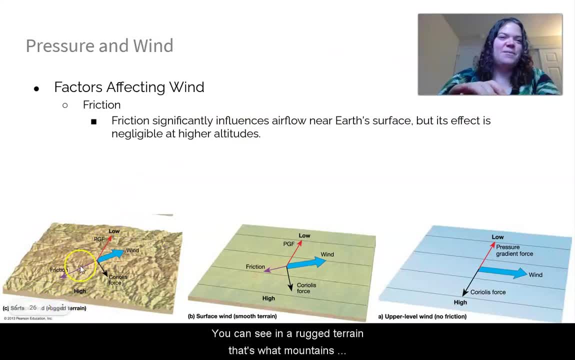 over here, um, you can see, in a rugged terrain that's with mountains, hills, valleys, rugged terrain. i see pgf is pointing from high to low. i see the coreos deflecting to the right and then i see friction pulling my wind backwards. so that's the purple line. so the purple. 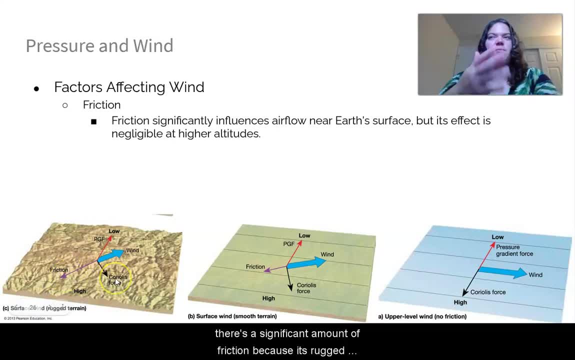 line pulls my wind backwards and there's a significant amount of friction because it's rugged terrain, so my wind is slow. right then if i'm on a smooth surface like grassland right or an ocean- um, ocean's a bad example- we'll stick with grassland. so grassland- we see pgf is still pointing from high to low or else is still to. 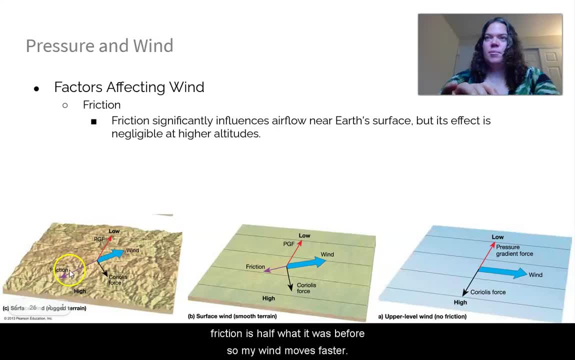 the right northern hemisphere, but the friction is half what it was before. so my wind moves faster and then, as i move to the upper level where there is no friction, we point again from high to low, and then the coreos is to the right and the wind moves parallel to the ice bars. 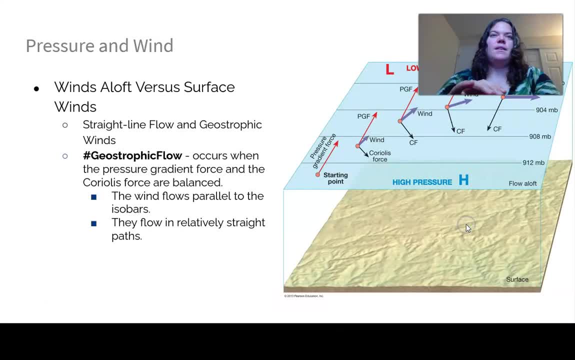 tada. so when we have these straight line flow, we end up having something called geostrophic flow, which occurs when the pressure, gradient force and the coreos force are actually in balance. so the wind flows parallel to the isobars and they flow in relatively straight paths. 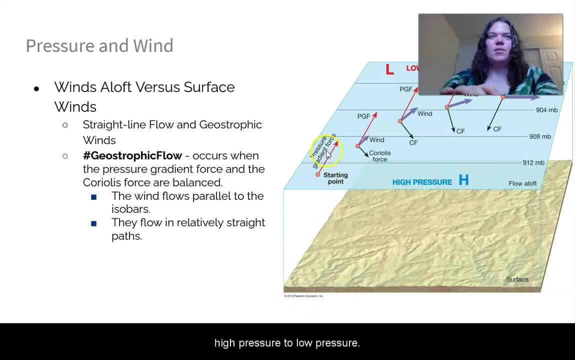 so here we see, if we start towards the high pressure, pressure gradient force pulls it towards the low pressure, and then the choreo starts tugging it this way. so the pressure gradient wants to go that way, and then the coreos tugs it this way, and then they end up in some kind 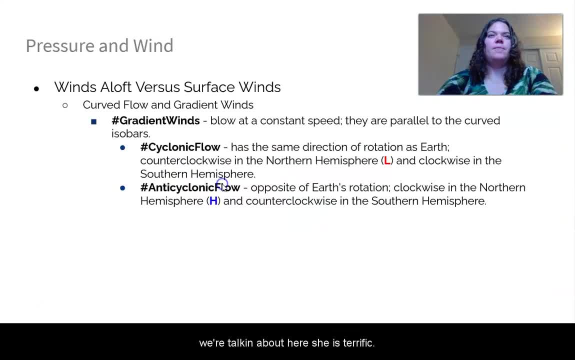 of balance, and that is what we're talking about about here, geostrophic flow. and then there are gradient winds. they blow a constant speed, they are parallel to the curved isobars and cyclonic flow has the same rotation as the earth. it is counterclockwise in the northern hemisphere and clockwise in the southern hemisphere. 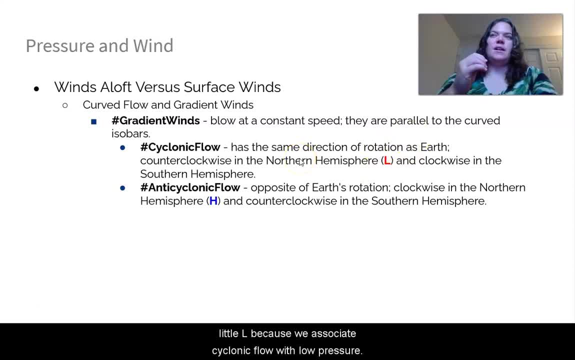 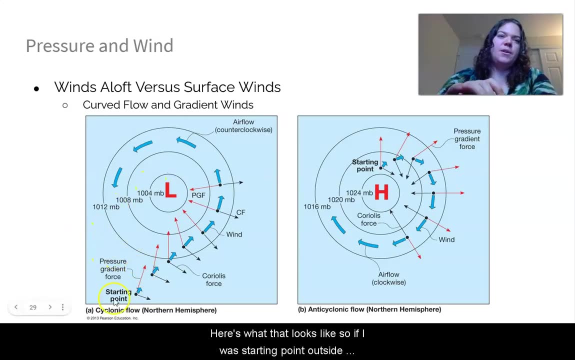 again there's my little l because we associate cyclonic flow with low pressure um. anti-cyclonic flow is the opposite of the earth's rotation, so it's clockwise in the northern hemisphere and then counterclockwise in the southern hemisphere. here's what that looks like. so if i have a starting, 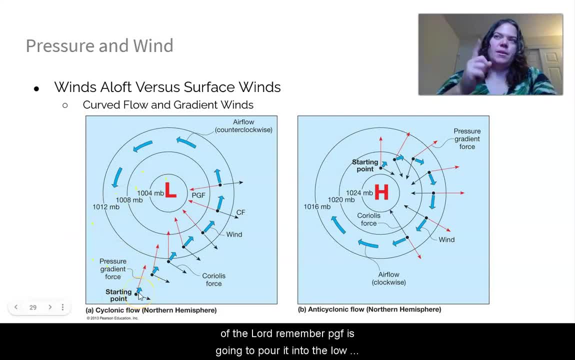 point outside of the low. remember, the pgf is going to point into the low, so it's pulling it this way. coriolis pulls it to the right, and then again they reach some kind of balance, and so we get this counterclockwise flow. that's where that comes from. 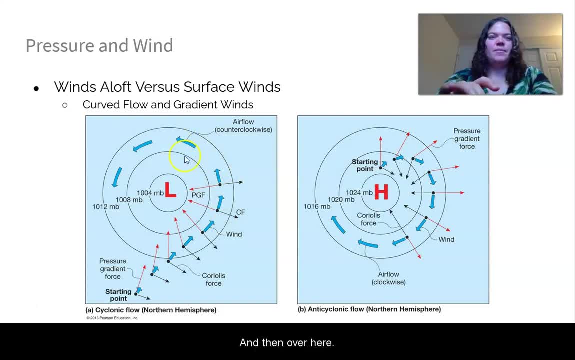 again northern hemisphere. okay, and then over here i see there's a starting point from the middle of the high. i don't know why it's not blue, but whatever. so we have a starting point from the center of the high pressure and then it's pulled outward by the pgf, because it always points from. 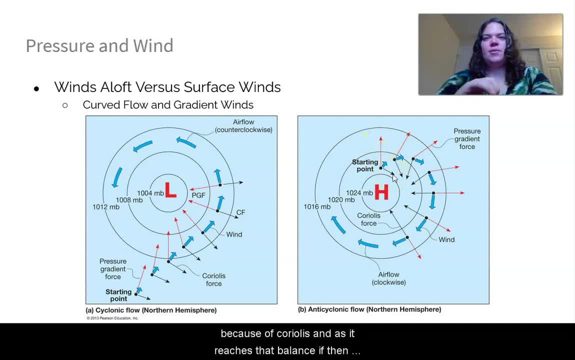 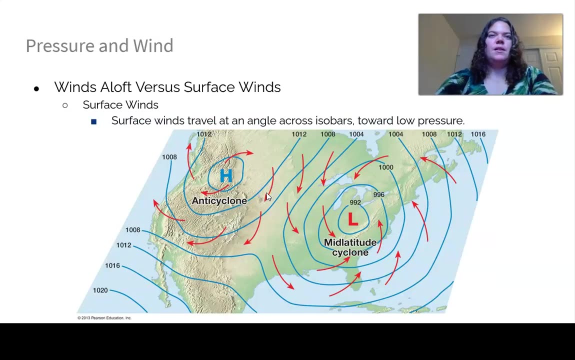 high to low, and it's curving to the right because of coriolis, and as it reaches that balance, it then flows clockwise around the high pressure. so that's where those directions come from. is the pgf and the coriolis interacting with each other in the wind? so this is what it really looks like. 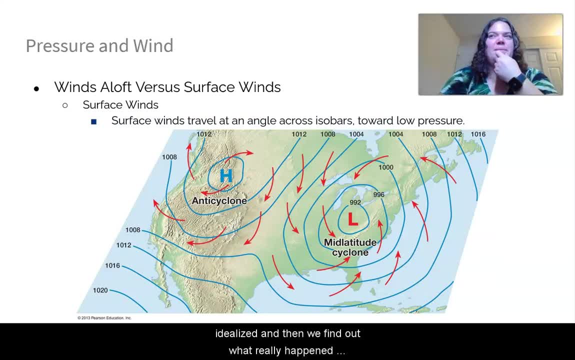 because everything's idealized and then we find out what really happens. um, no, seriously. so surface winds actually travel at an angle across our isobars because of friction. so friction at the surface makes it turn about 30 degrees across the isobar. so we see, for the mid-latitude cyclone, the 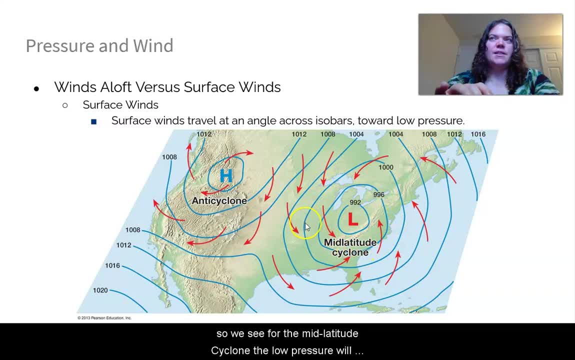 low pressure will have winds that are counterclockwise and also inward, okay, so they kind of cross and then they go inward and the anti-cyclone is the opposite. they flow clockwise- let me get it right- and outward, so clockwise and outward for the anti-cyclone. so we use something called pressure tendency. 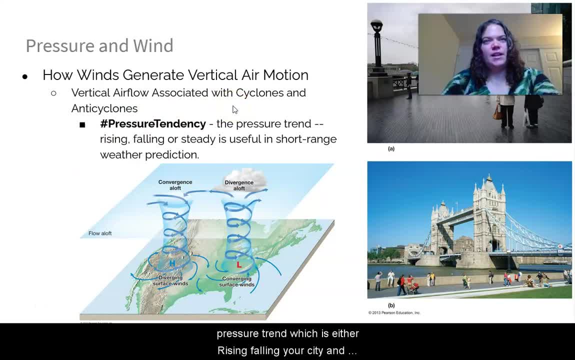 or the pressure trend, which is either rising, falling or steady, and then there's variations of that to short range weather forecast. okay, so if i have what we have here- converging surface winds, which i just told you are associated with low pressure, so it kind of spins up like a dyson vacuum cleaner, not a sponsor, and we get divergence aloft. so this spinning 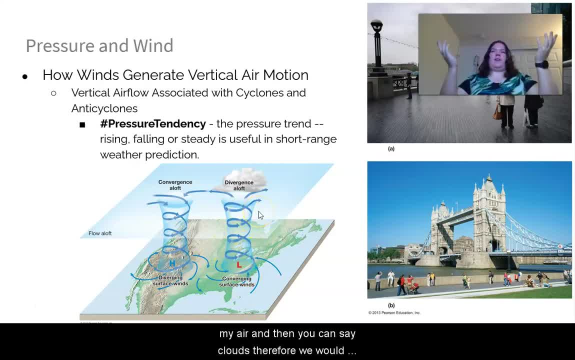 action actually lifts my air and then you can create clouds. therefore, we would associate the low pressure with the top picture. right, because i have clouds here. it's raining, we've had lifting, we have clouds for and we have precipitation, so the opposite is also true. if i have 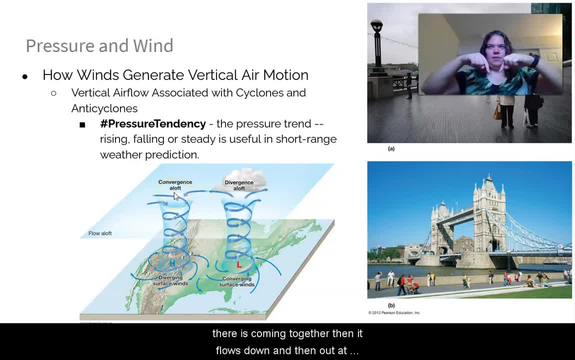 a winter, we get these high as we get into a gradient, and then the other thing is that if you'll look at the top picture, it's like a dark spot and you're like, okay, but we're doing anika, and когда we start to adopt, 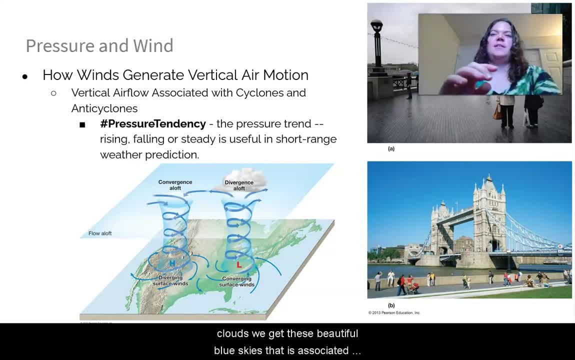 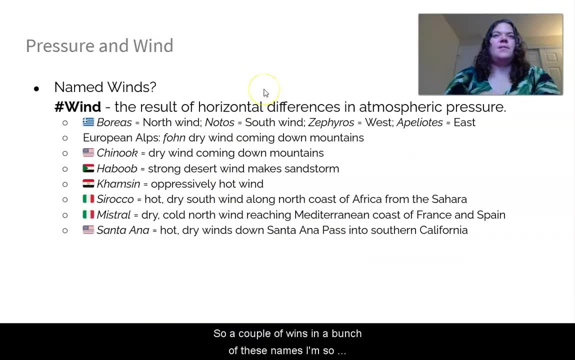 it. it's like i'm coming from a fall, so we get like a gradient again and then we get what's called a burst here and we get the energy. it's like all the energy that is going to flow in the bottom, so we get these beautiful blue skies. that is associated with high pressure. okay, so a couple. 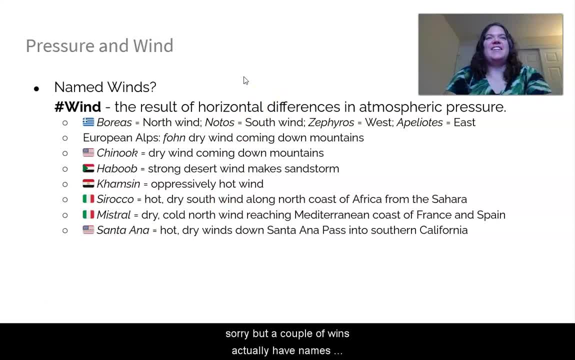 of winds. actually, i'm going to butcher these names. i'm so sorry, but a couple of winds actually have names associated with them and remember, wind is the result of horizontal differences in atmospheric pressure. the pressure gradient force is what causes wind to happen. okay, so in greece, like my 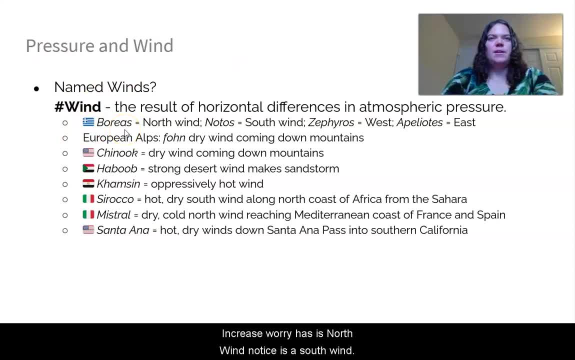 little flag. so in greece, boreas is a north wind, notos is a south wind, zephyros is a west wind and apeliotes is a east wind. i think i'm doing a bad job, but anyway, um, please don't hate me. the european alps has something called a fjorm dry wind come down. 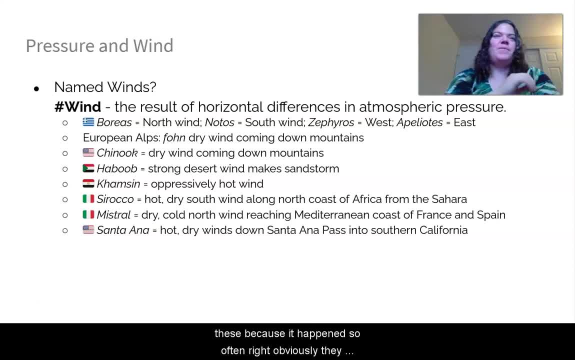 from the mountains and they name these because they happen so often. right, obviously they get different names, but they're not the same thing, so i'm going to name these because they happen. right, obviously they get different names, but they're not the same thing, so i'm going to name these. 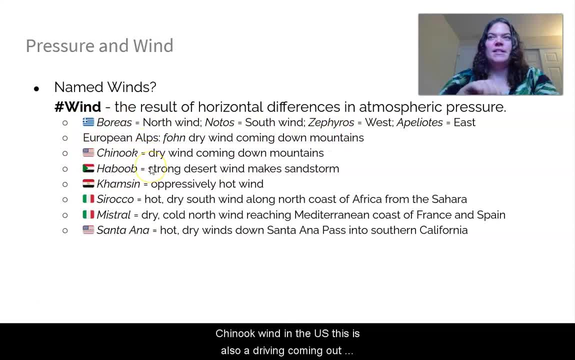 all the different winds in greece, but um, there's a chinook wind in the us. this is also a dry wind coming down from the mountains. the sudan has a haboob um wind, which is a strong desert wind that makes a sandstorm. so you get this massive sandstorm from this kind of wind, and then there's a. 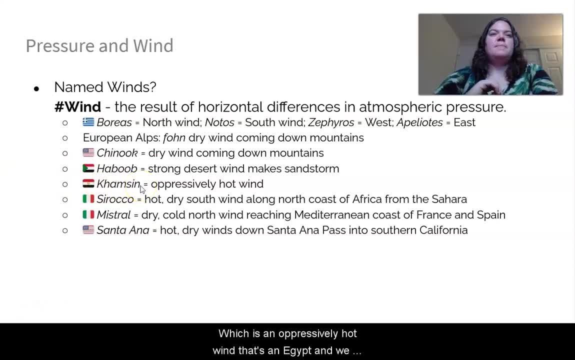 oh, cause scene on scene, which is an oppressively hot wind. that's in egypt. then we have a cold wind. that's in egypt. and then we have a cold wind, that's in egypt. we have a soroko, which is a hot, dry south wind coming from the north coast of africa. 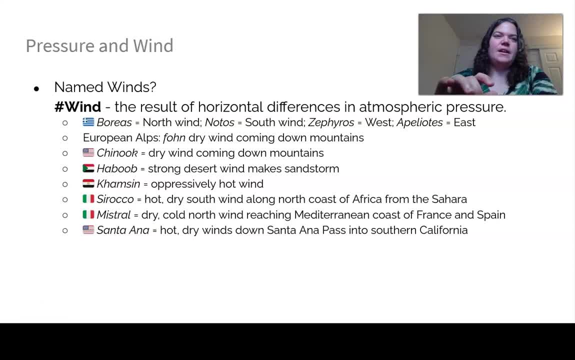 from the sahara that is into italy, and a minstrel, which is a dry, cold wind from the north, reaching the mediterranean coast of france and spain, also italia, italia, italy, sorry guys. and um, the us has santa ana winds, super famous, hot, dry winds, coming through the santa ana pass into southern california. 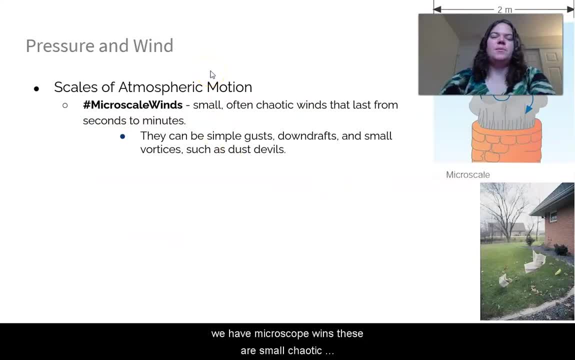 so let's do scales of motion really quickly. so first we have micro scale winds. these are small, chaotic winds that last from seconds to minutes. they can be simple gusts down drafts, small vortices, like on the side of a building which you see here, small vortices and dust devils. so here's. 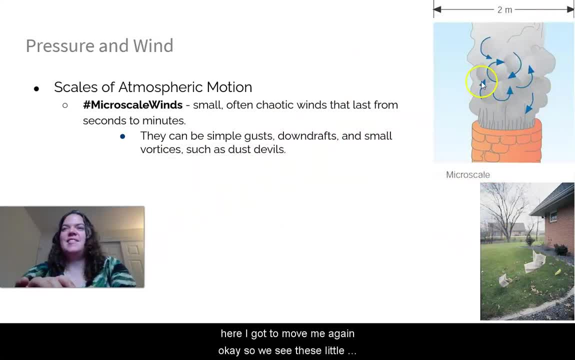 micro scale here. i gotta move me again over there. okay. so we see these little turning arrows here inside this chimney. on a two meter scale that's considered a micro scale wind and then we have a mesoscale wind. then as i move up in the scale, i reach mesoscale winds. these last for minutes to 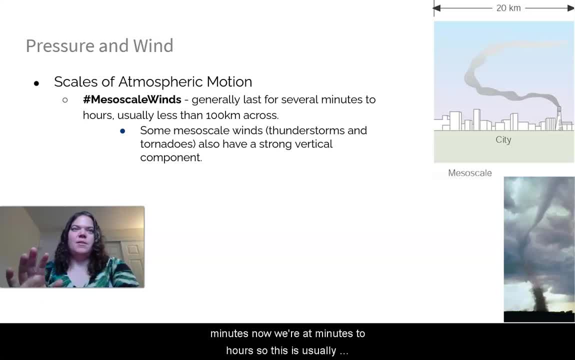 hours, so we were at seconds to minutes. now we're at minutes to hours. so this is usually less than 100 kilometers across, so we're talking about the size of the city. so there's that chimney. we were just looking at right, the smokestack, and now it's inside the whole city, so we zoomed out. 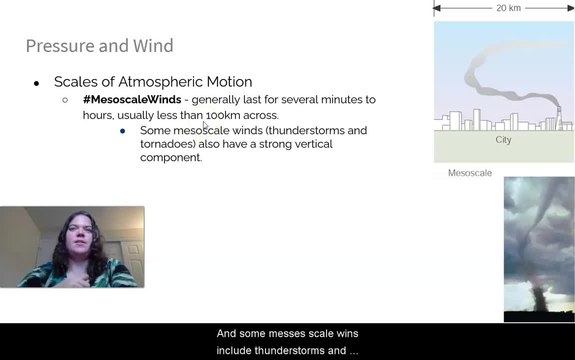 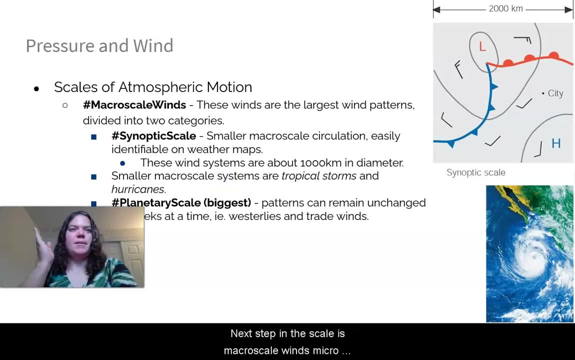 and some my mesoscale winds include thunderstorms and tornadoes, which i have a picture right here, and they have a strong vertical component to them. next up in the scale is macro scale winds. so we go micro, meso, macro, so they're getting bigger, we're zooming out. so that city we just looked at is this. 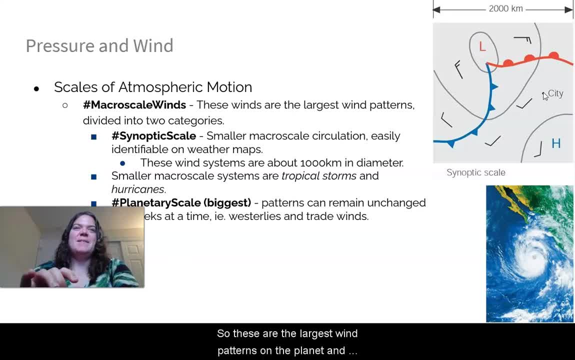 dot right here, so we really zoomed out a lot. um so, these are the largest wind patterns on the planet and they are divided into two categories. the smaller of the two is synoptic scale. these are winds easily identifiable on weather maps, like the one on the right, and they're about a thousand. 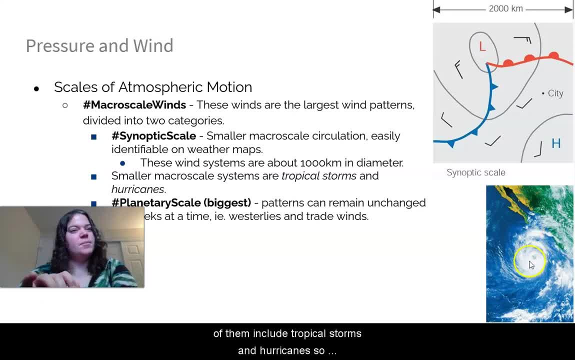 kilometers in diameter. some of them include tropical storms and hurricanes, so those are actually synoptic scale storms, and then the planetary scale is the biggest, and these patterns can remain unchanged for weeks at a time. so again, we went from like seconds, minutes, hours, days. now we're at weeks. so we're really, really zooming out. so these are the westerlies in the trade. 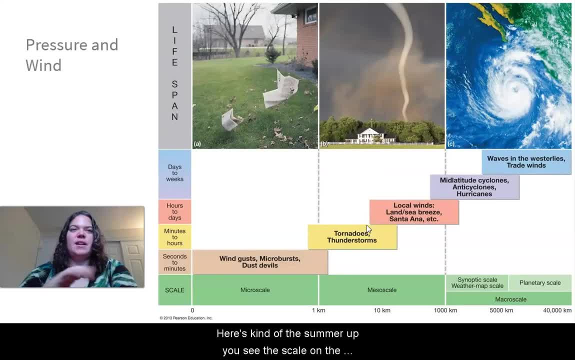 winds, which we'll talk about later in class. so here's kind of a sum up. you see, the scale on the bottom is distance and then the scale on the left is lifespan in um time. so we see there's our wind, gusts, microbursts and dust devils are in the micro scale for seconds to minutes. then we see those. 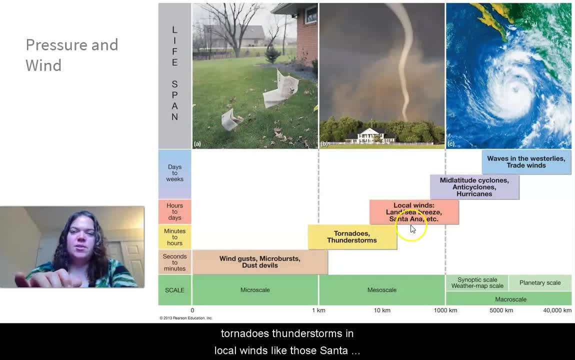 tornadoes, thunderstorms and local winds like those Santa Ana ones. we just talked about our mesoscale and they last from minutes to hours or maybe even days. and then synoptic scale, which is part of the macro scale, the smaller end, that's weather map scale. you see mid latitude, cyclones, anti-cyclones and hurricanes. cyclones and anti-cyclones- we just 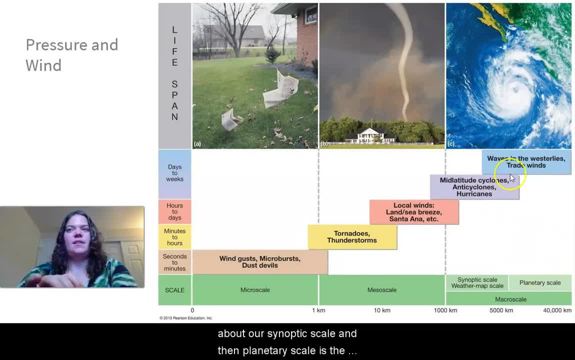 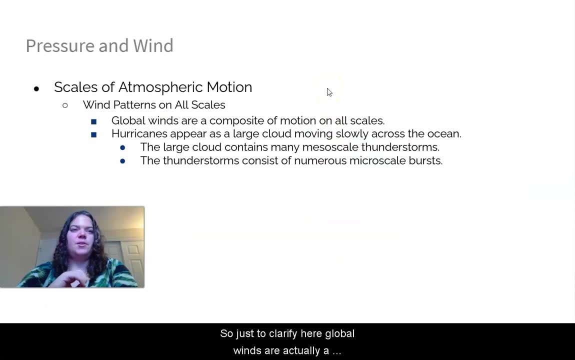 talked about our synoptic scale and then planetary scale is the trade winds or winds in the westerlies. so just to clarify here: global winds are actually a summation of all the smaller scales. so, for example, a: if we look at a hurricane, it's a big, large cloud, right, but the large cloud actually contains many. 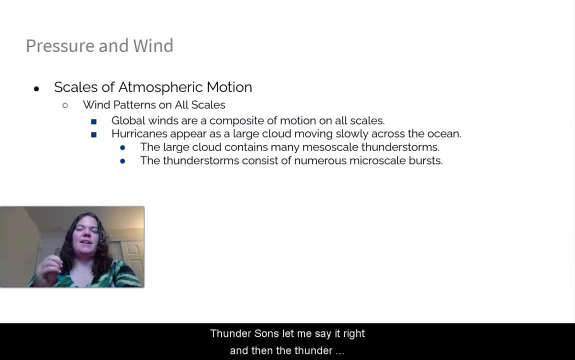 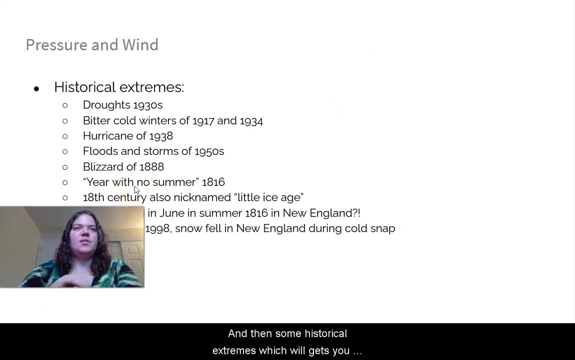 micro, um mesoscale thunderstorms, let me say it right, and then the thunderstorms have micro scale bursts in them. so it's like a summing up of all the energy, all the scales, to get that big storm. that's the hurricane, okay, and then some historical extremes, which we'll get to more in another lesson. 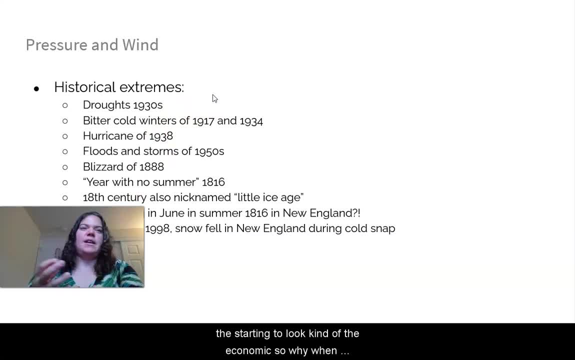 but we had droughts in the 1930s. just going into like kind of the economics of why wind, storms and storms matter to begin with, um, we had the bitter, cold winters of the night 1917-1934, the hurricane of 1938. we have floods. 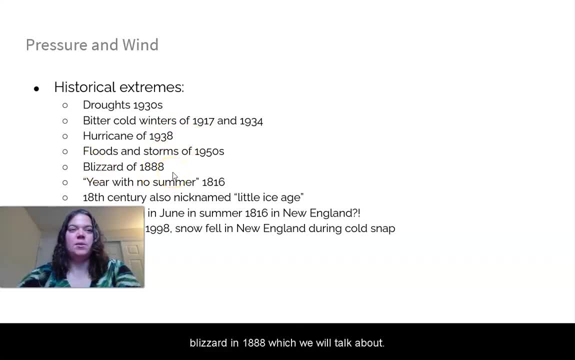 and storms in 1950s. there was a big blizzard in 1888, which we will talk about, and then there was a year without a summer in 1816, also known as the little ice age, and snow actually fell in June and summer 1816 as well. plus, there was a record heat in 1998. we will talk about why that is a little bit. 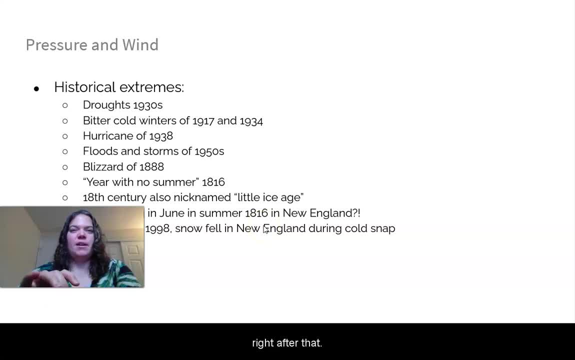 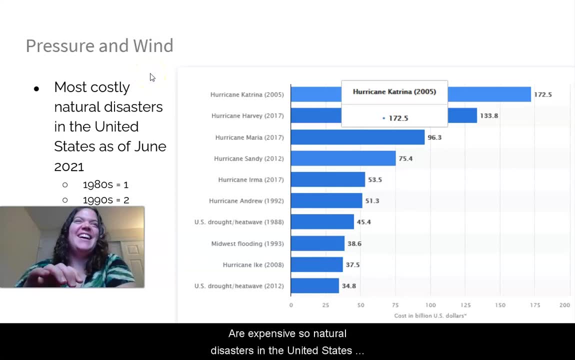 later, and snow fell in New England during a cold snap right after that. why do we care? because they're expensive, basically. so natural disasters in the United States are again focusing on the United States now. um as of June of this year, I found this top 10 chart. 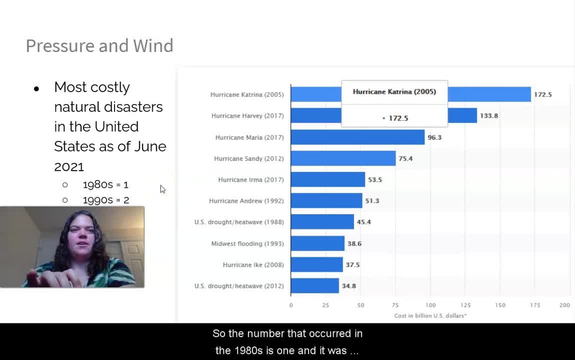 so the number that occurred in the 1980s is one, and there was a US drought in heat wave right here and it caused 45.4 billion dollars in damage, that's B billion B as in boy, and 1990s had two. 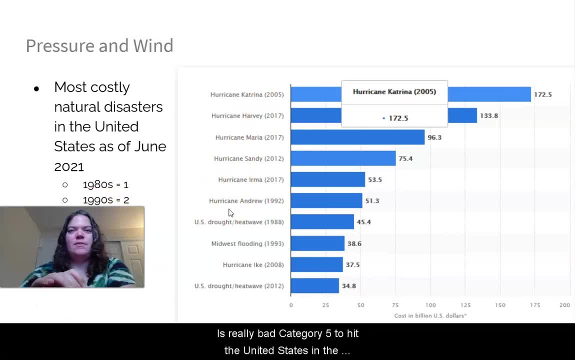 swarms. you see, Andrew, it was a really bad category 5 to hit the United States and the Midwest flooding of 1993, which we'll also talk about, um vomit, yeah. so, just like we said before, all thesechwad flooding, for ought to see these two storms again, and not the near one, but quite a bit of a relief to be able to be able to keep your